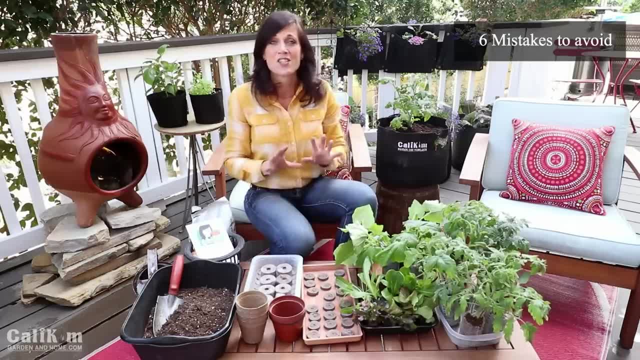 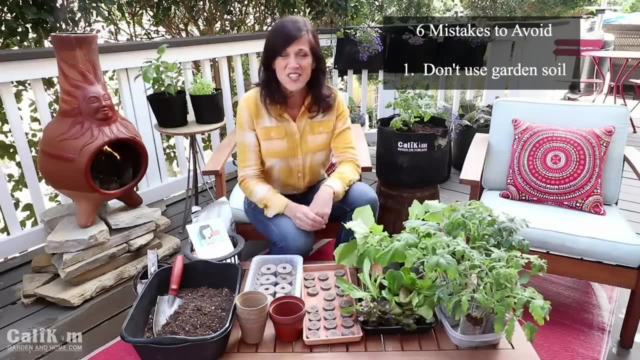 thing to avoid when you're starting from seeds indoors is: don't use your garden soil. So don't go out in your garden, just dig up a pile of soil and think that that's going to be okay for starting your seeds. Your garden soil is just too heavy, gets too compacted in these little containers. 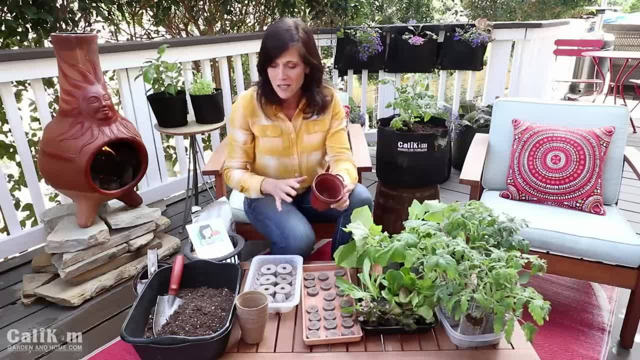 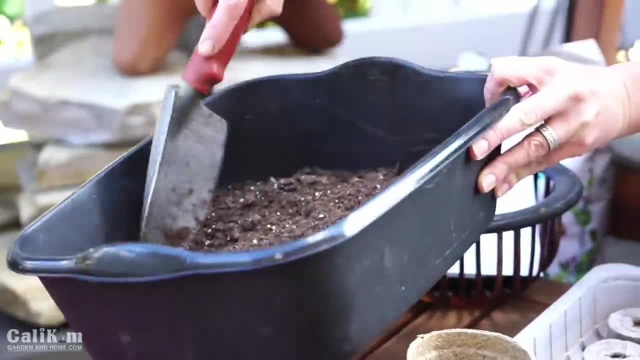 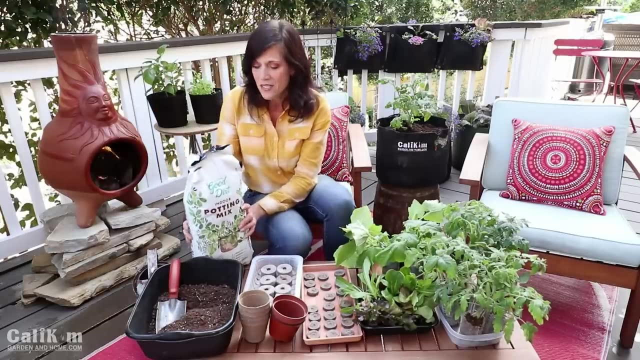 it's not light and fluffy enough for germinating seeds, So what I've got in my little bin here is some nice, light and fluffy seed starting mix. I love to use this Good Dirt Indoor Potting Mix. This is the best indoor potting mix I found to use for my seeds. It's nice and light. 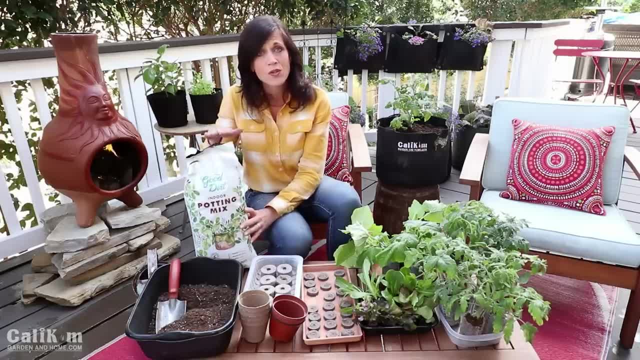 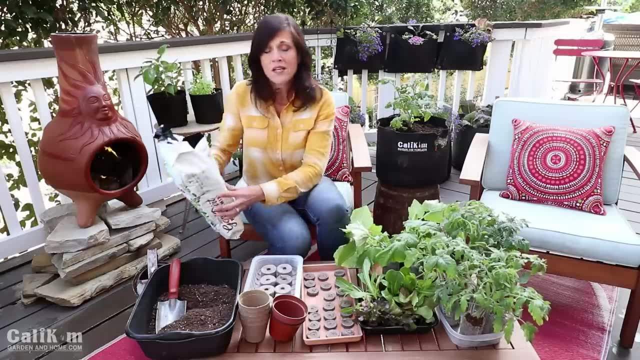 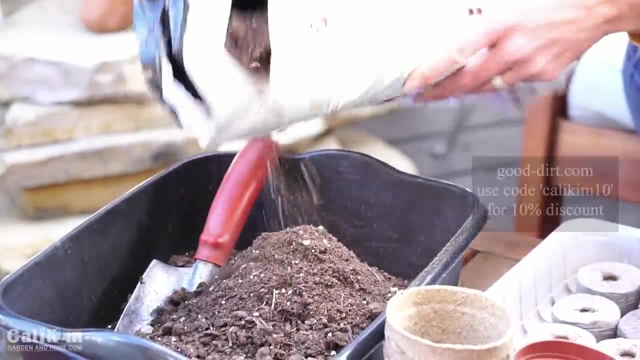 and fluffy, and this is now available at your local Target store. So check online at targetcom, pop in your zip code and see if it's available at your local store. You can also pick some up at good-dirtcom and use my code, KALIKIM10, for a 10% discount. So we're going to start some seeds. 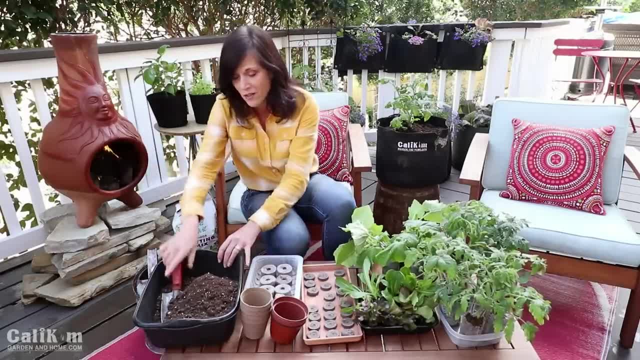 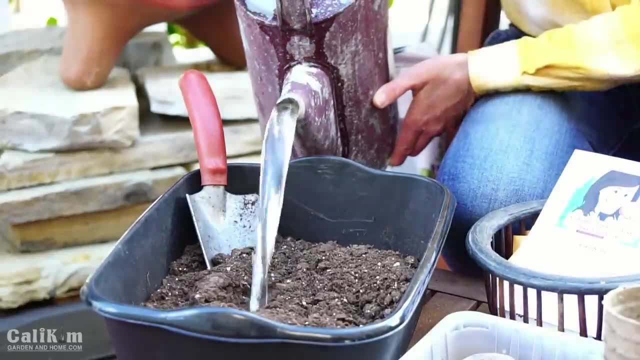 here. The first thing I'm going to do is just pour in my potting mix into my little container here And I'm going to pre-moisten my potting mix before I plant my seeds. Pre-moistening your potting mix is super, super important, because you want your seeds to get off to a good start and 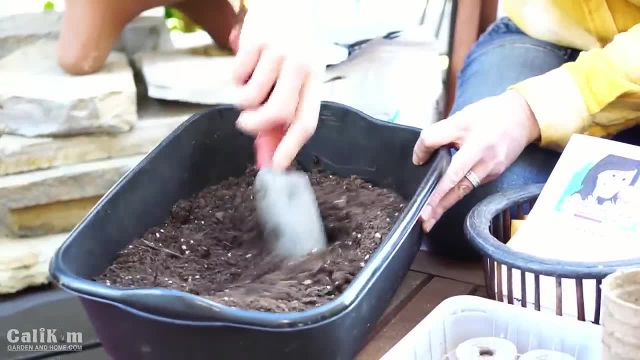 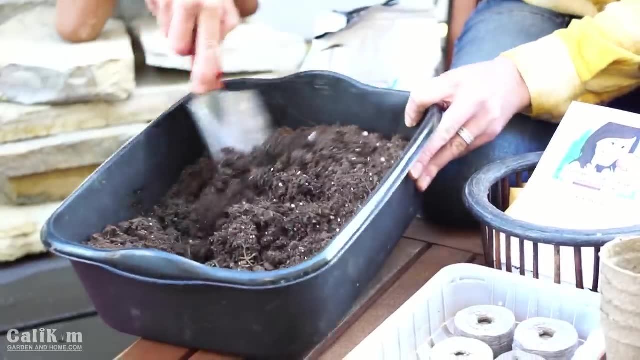 have all the water they need to start growing right away. So I'm just going to pour some water in here and then mix it around until it's about the consistency of crumbly brownie mix, And it is really important to have a really good, high quality seed starting mix. 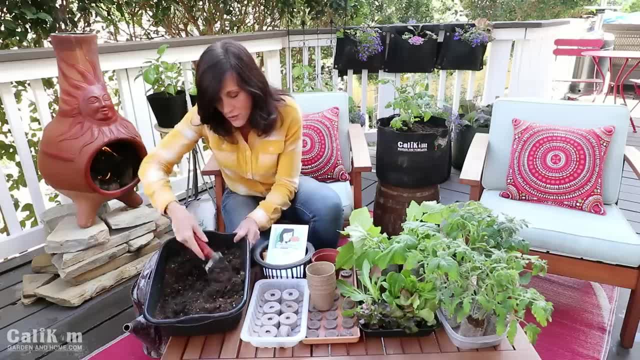 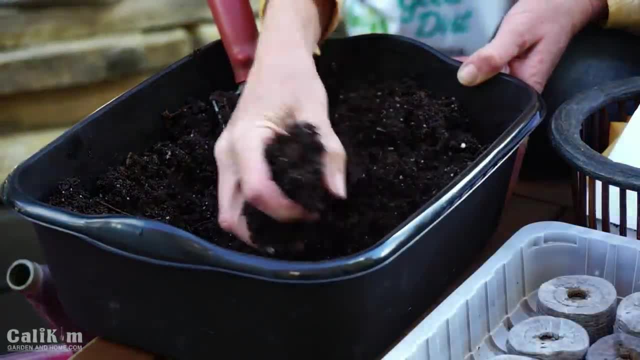 because it'll have some nutrients in it that'll help your seedlings get off to a good start and grow until they're ready to go out in the garden. Okay, you can see this is about the right consistency. Looks kind of like crumbly. 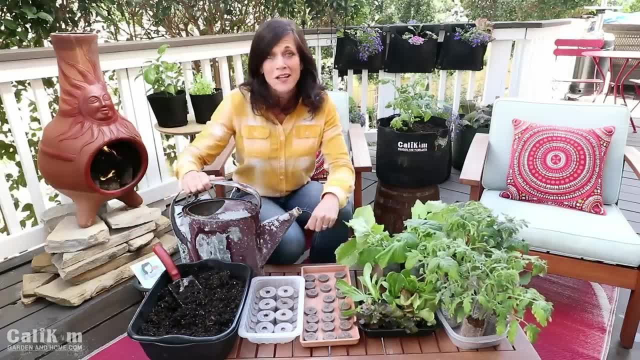 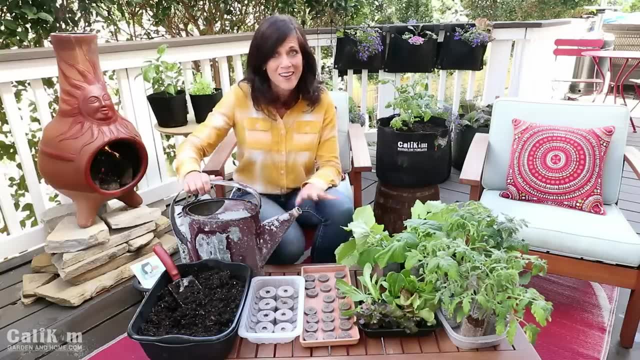 brownie mix. So we've got our soil ready. now we're going to get our peat pellets ready. Now, if you've never used peat pellets, you're in for a treat If you have kids. grab your kids to watch this part, because they are going to love it. So we've got here a larger size peat. 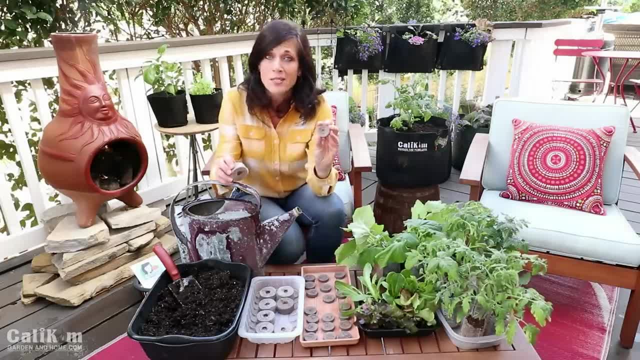 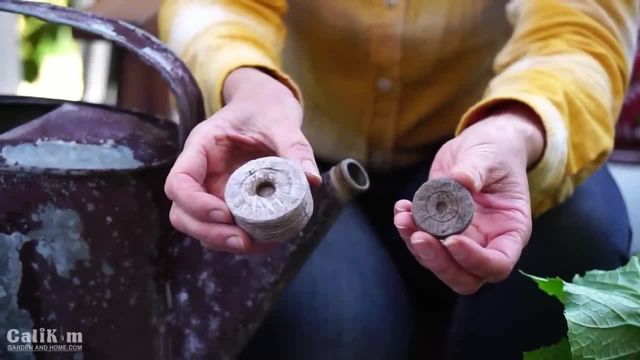 pellet for larger size vegetables and a smaller size peat pellet for smaller size vegetables. Now, these are super, super fun. They're just little compressed blocks of soil And we're going to add some water here and they're going to expand in a couple of minutes and we're going 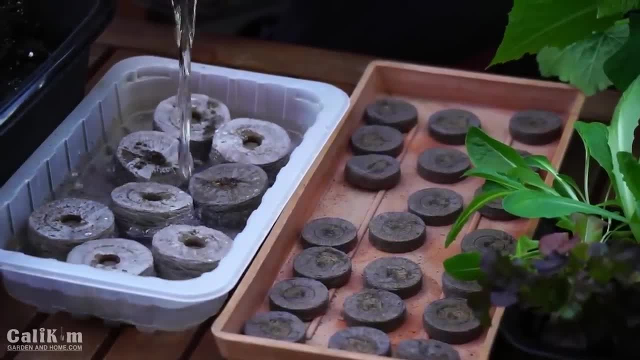 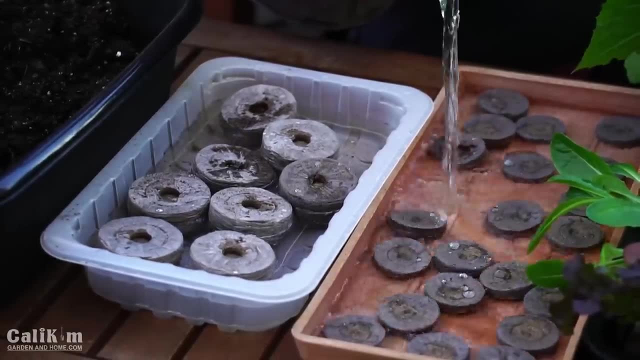 to be able to plant our seeds right in these pellets. Now, I love growing in pellets because it's super, super quick. It's a no fuss, no muss way to grow. So if you don't want to make a mess in your house when you're starting your seeds, the peat pellets are definitely the way to go. 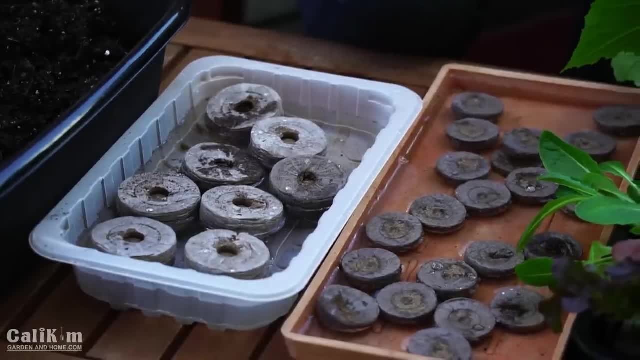 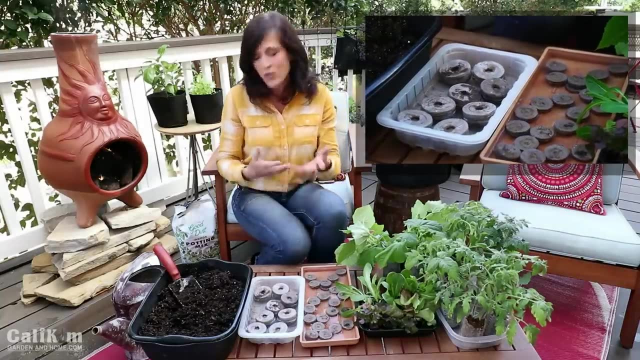 And I'll link everything in the video description below so you know exactly where you can find these products. So, while these expand, what we're going to do is talk about the seeds that we're going to use Now when you're starting seeds for your spring garden. 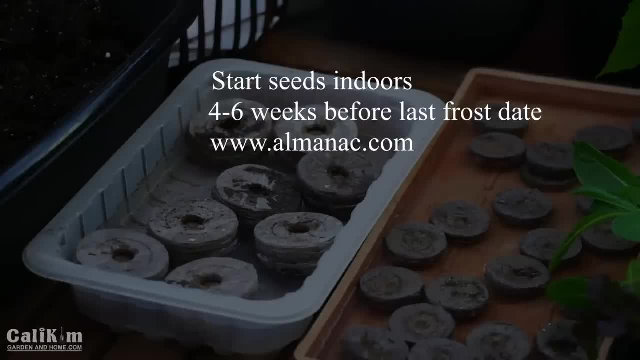 you're going to be planting some warm weather vegetables. You want to start your seeds indoors four to six weeks before your last frost date And you can find your frost date at FarmersAlmanaccom. Super, super exciting to get those beautiful tomatoes. cucumbers squash. 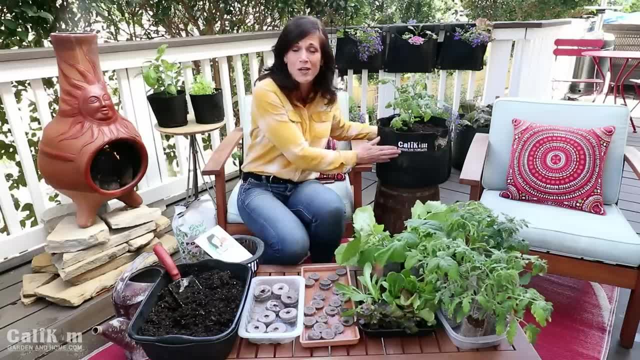 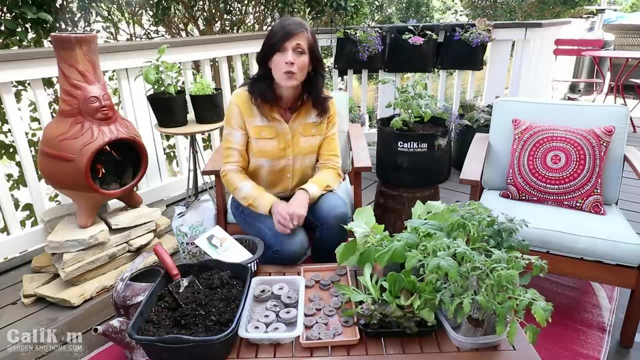 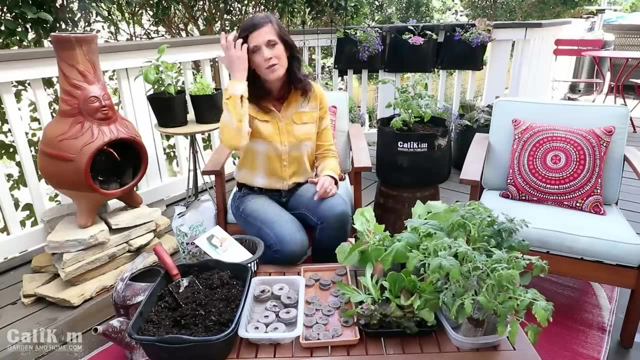 Look at this tomato plant here. This is a little tiny tomato that I've been growing indoors and it's already starting to develop a little teeny, tiny tomato. So it's going to be so exciting when the weather gets warm enough outside to have your own beautiful vegetables to plant out in your garden, harvest and eat a few months later. 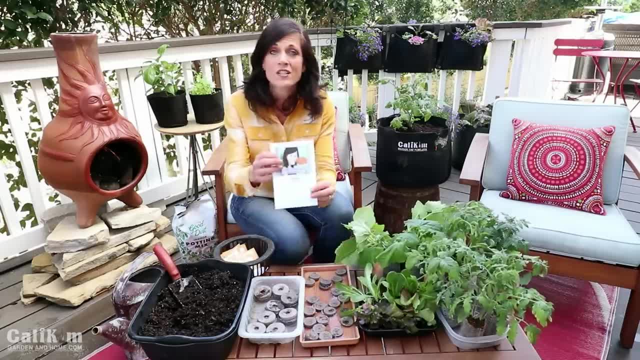 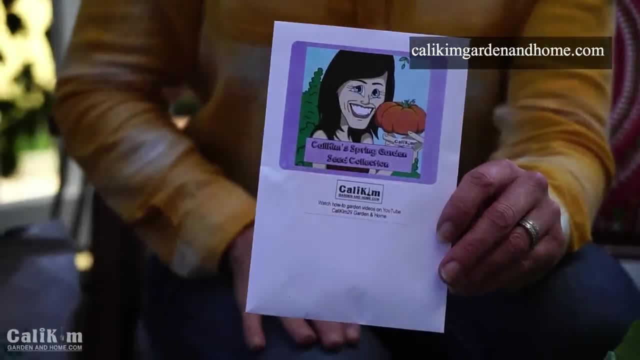 and bring in to feed your family. So we're going to be growing with my spring garden seed collection. You can get this on my website at CaliKimGardeningHomecom. It's got 12 varieties. It's going to help you get a basic garden started all in one nice handy. 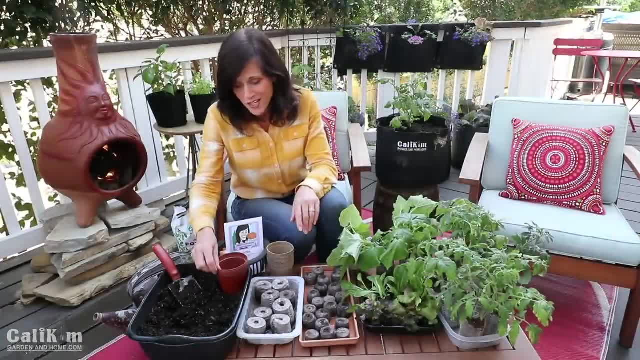 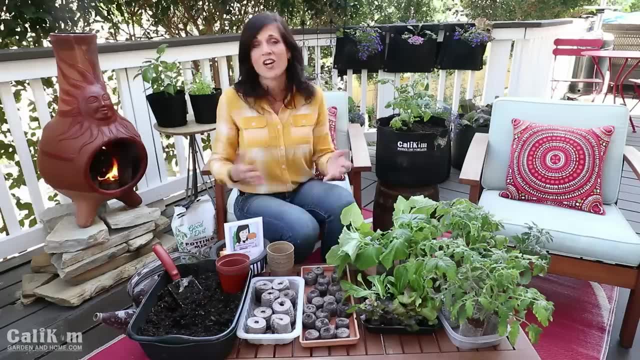 while we're waiting for our peat pellets to finish expanding, Let's get some seeds started here with the soil. So, first off, you don't need to worry about buying anything too fancy, any fancy containers. Just look around your house and see what you have around your house. You can use old 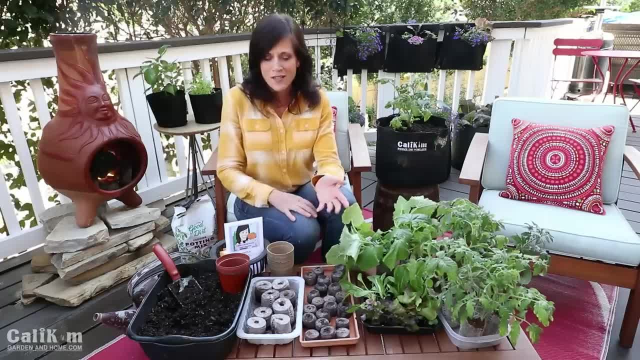 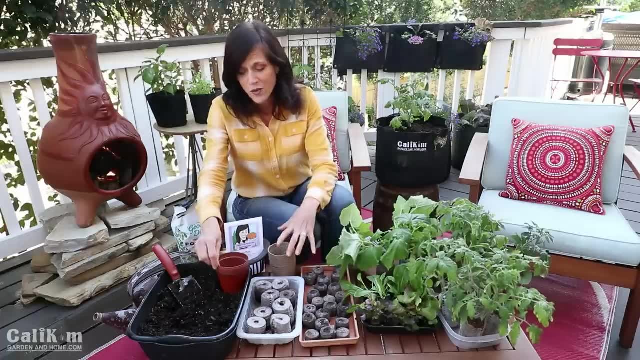 sour cream containers, old yogurt cups, even egg cartons. You can pick up some of these little recycled cardboard containers from your garden center or on Amazon. What I like to do is just recycle the little nursery pots that you get from the garden center when you buy transplants. 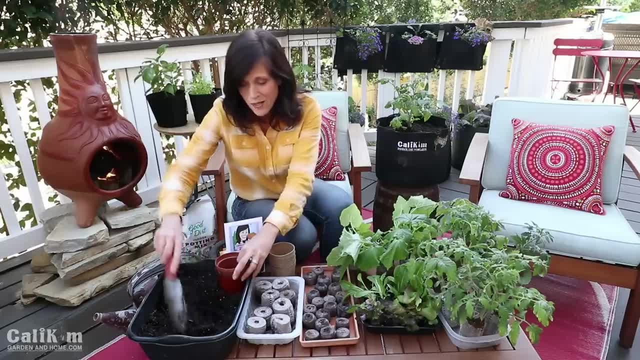 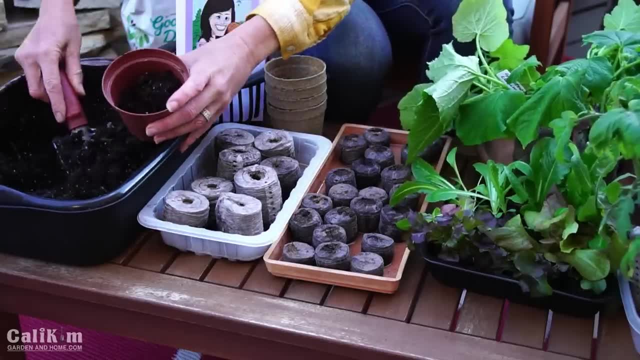 That way you're getting started totally free and on the cheap. So now that my soil is all moistened up here, what I'm going to do is fill up a couple of these little containers with soil. I'm going to fill them up all the way to the top And then I'm going to kind of pack them down just a little bit. 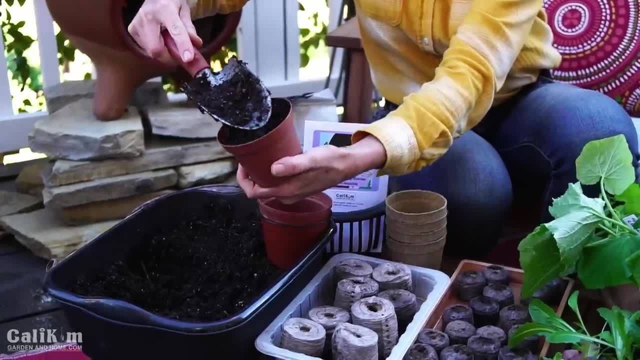 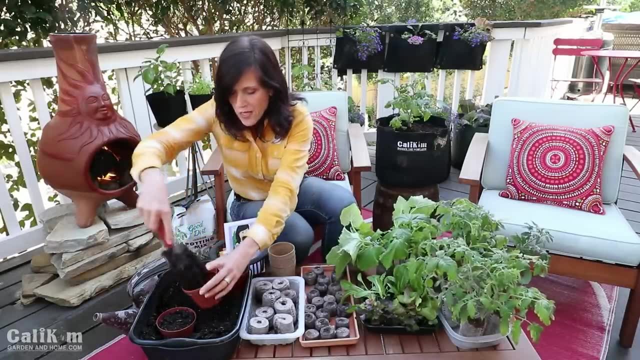 here with my shovel because I don't want any air pockets for my seeds. I want my seeds settling down in there nice and tight so that they have a really good germination rate. So I'll fill up a couple of these containers And in these containers we're going to plant some of these little 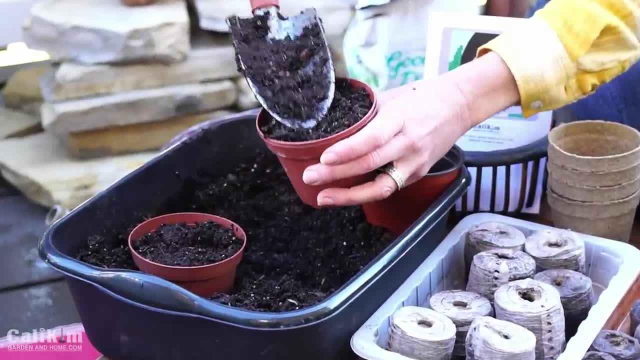 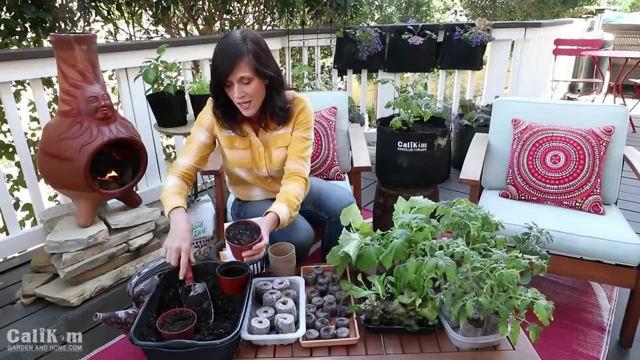 seeds that grow very, very quickly, And the reason why we're doing that in the cups with soil as opposed to the peat pellets is because they're going to outgrow the peat pellets really, really fast And we do need to grow these indoors for about four to six weeks. So we want to try and 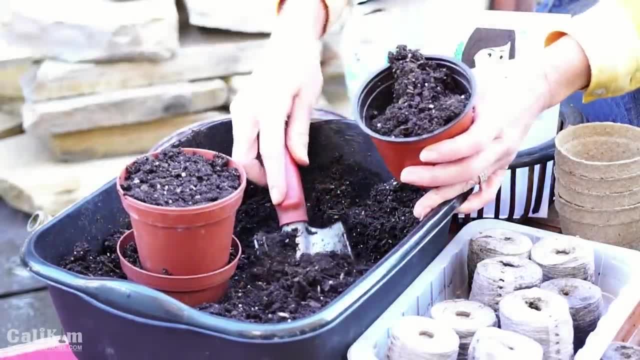 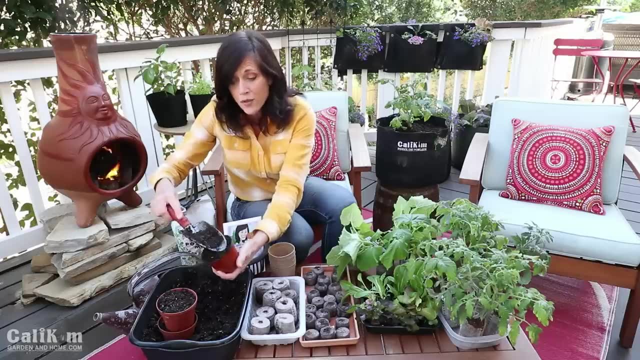 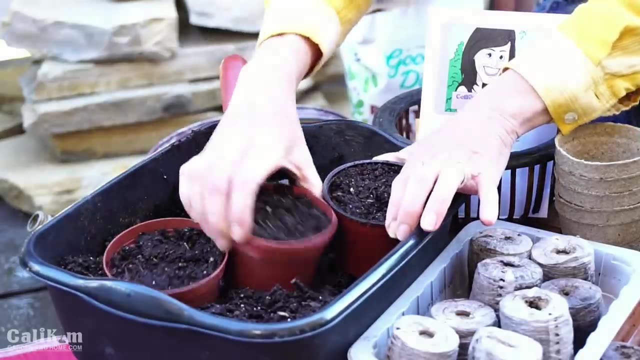 avoid transplanting them again while they're indoors, So I'm going to start them off in a larger container. So remember, we're avoiding mistake number one: We're not using garden soil. We're going to use a very nutrient-dense seed starting mix here. So I've got my cups with soil. 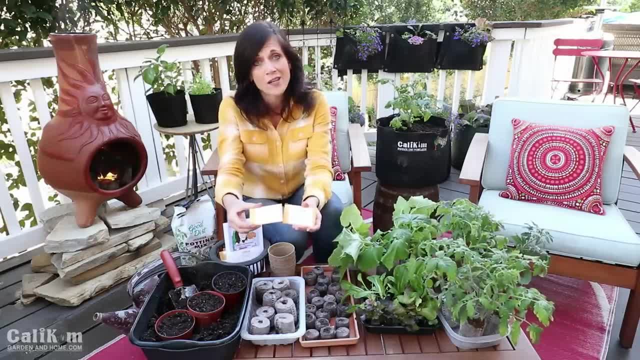 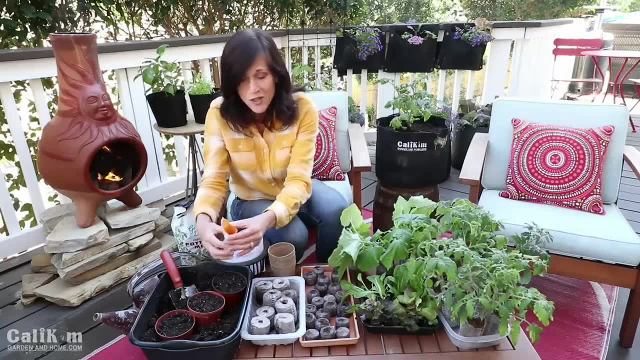 filled up And in these we're going to plant the Market More cucumber and straight necked yellow squash seeds from the Spring Garden Seed Collection. So first off, let's go for the straight necked yellow squash. I don't know how many of you love squash as much as I do, but we 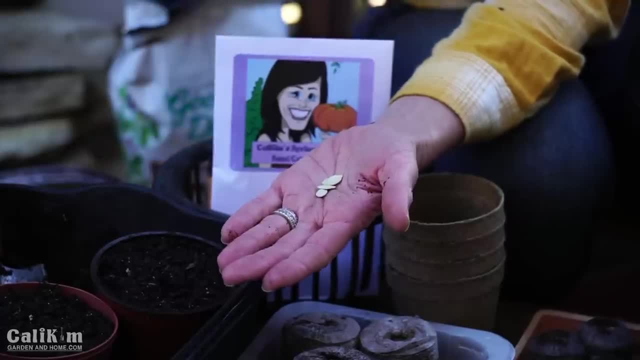 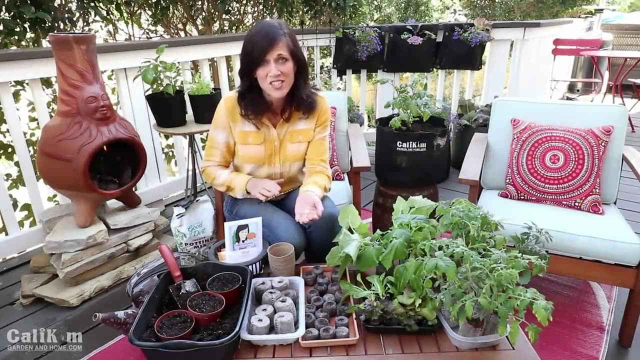 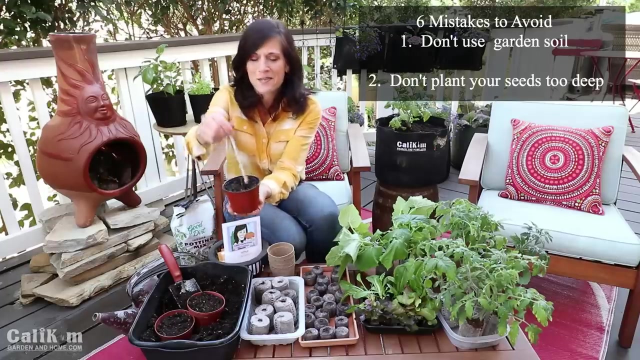 absolutely love harvesting it in the summertime and then grilling it up or roasting it in the oven. It's so, so tasty. One mistake to avoid when starting your seeds indoors is: don't plant your seeds too deep. A lot of people make the mistake of poking a hole in the cup that goes all the way down to the 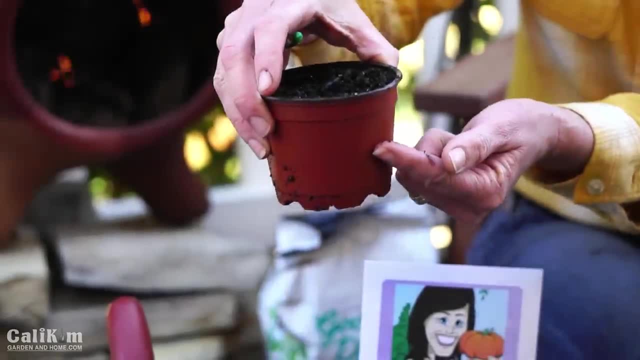 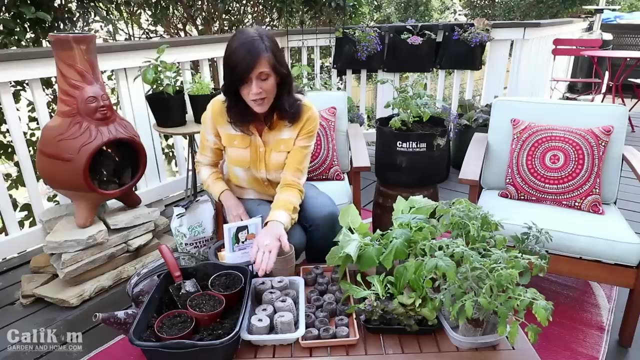 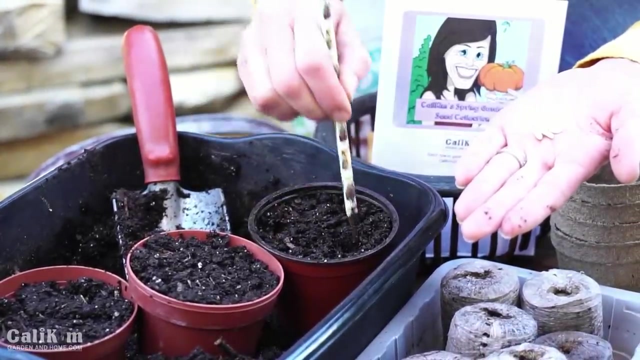 bottom, And then your seed drops way down here and it's way too deep to germinate. So the general rule of thumb is to plant your seeds about twice as deep as they are wide. So for these squash seeds here, I'm going to poke maybe a half-inch hole here in my cup And I'm actually going to 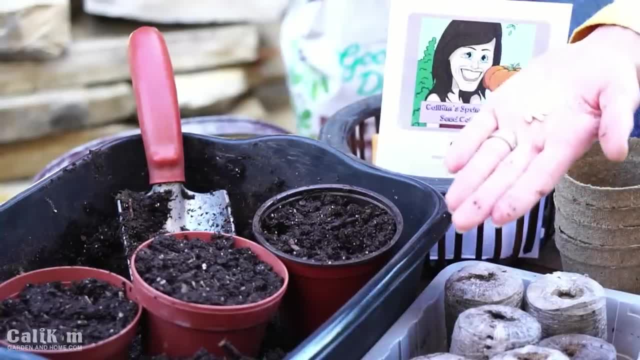 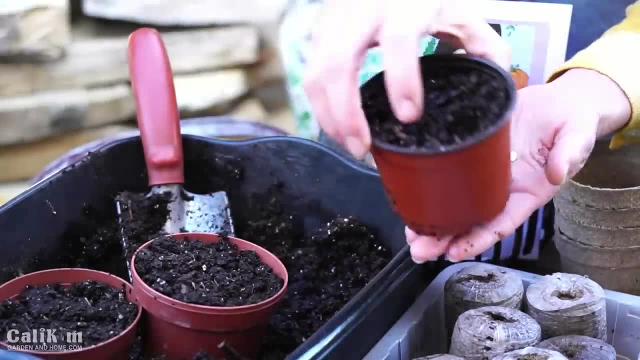 plant a couple of seeds. I don't want to just plant one seed, because that way, if that one seed doesn't germinate, then I'm out of luck. So I poked my hole about a half-inch deep. I'm just going to poke my seed. 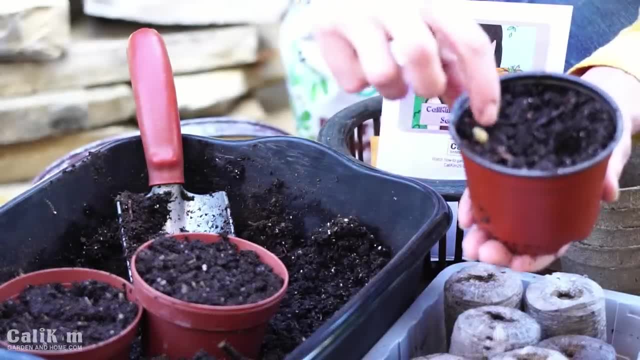 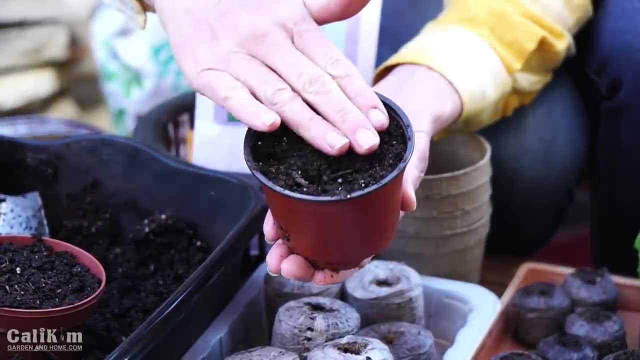 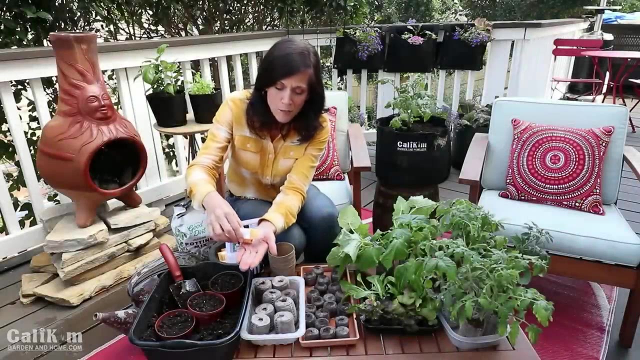 there down in the hole, both of my seeds, and then just lightly cover it up with soil And then just very gently tamp it down so there's no air pockets And that way we get a really good germination rate. So I'm going to do the same thing with my Market- More cucumber seeds. Now, I don't know about you. 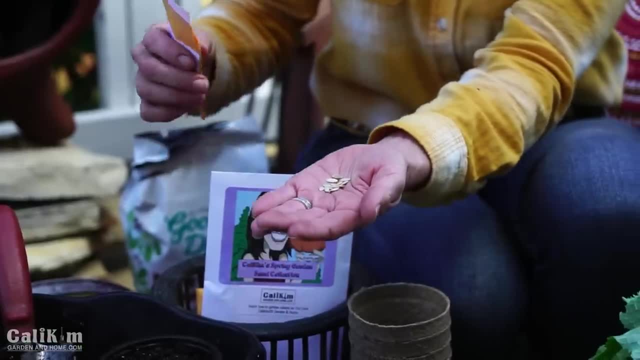 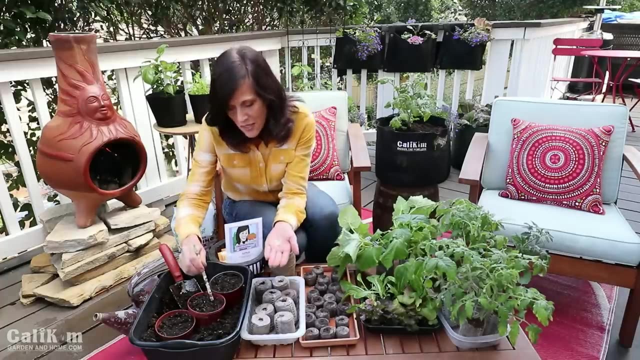 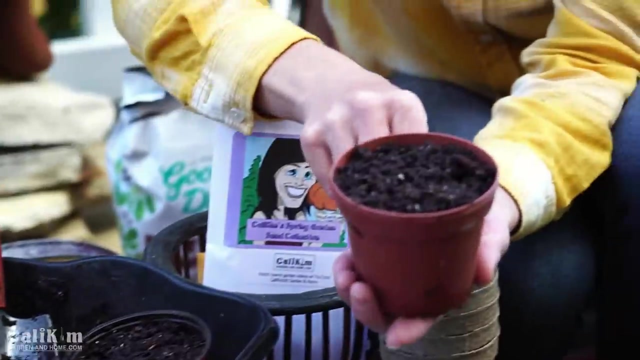 guys. but I absolutely love fresh cucumbers And it's so hard to find a good one in the grocery store. but they're super easy to grow, So why not grow your own right? So we'll do the same thing here with the Market: More cucumber Poke. just a small little hole here in my cup, drop in a couple. 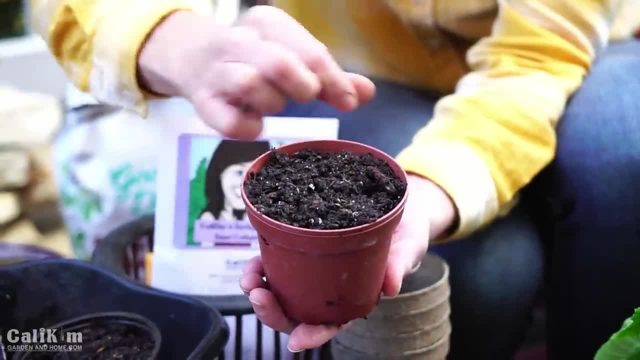 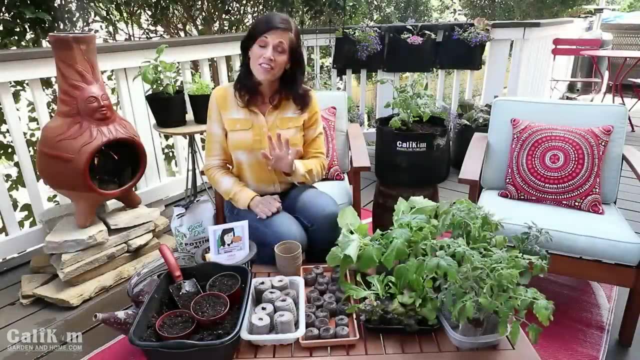 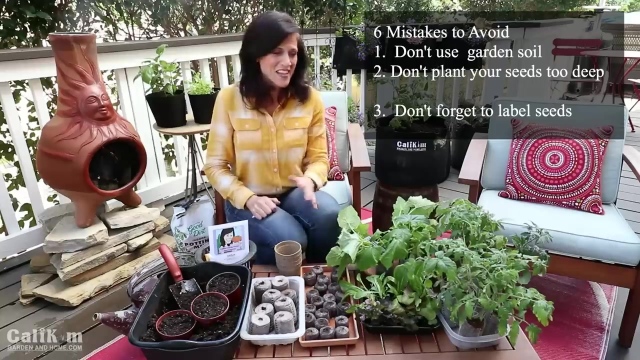 of seeds. I think I'll plant one more here. Cover them up, tamp it down and we are ready to go. So what you should do when starting your seeds indoors is: don't forget to label them. I am notorious with this. I have all these plants and I don't have a single label on either one of them. 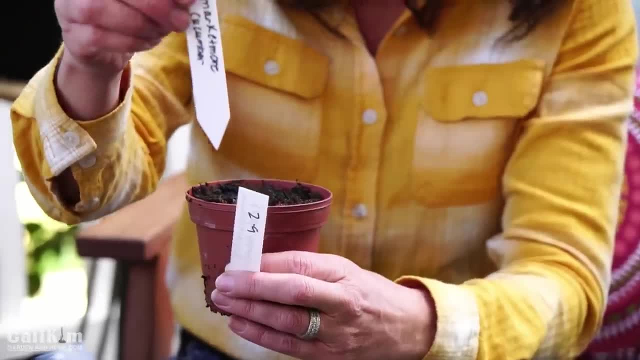 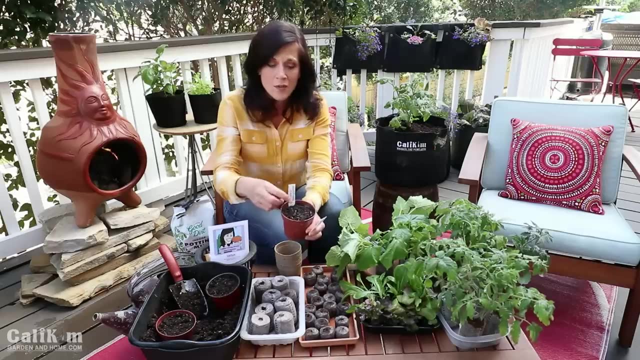 So we're going to label the seeds we just planted- This is the Market More cucumber- and I also like to put the date on the back, so I don't forget when I started them. So we're just going to pop this right here in this container with soil and label the other one, the straight-necked yellow squash. 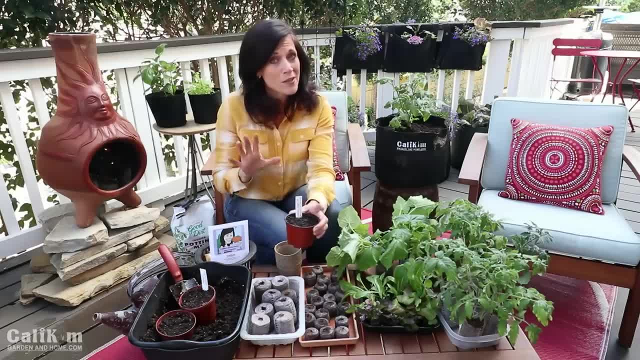 Because a lot of the seeds that you plant when they come up they're the same And if you're a beginner, you're not going to know the difference between a squash seedling and a cucumber seedling. So this way you know exactly what you're planting. 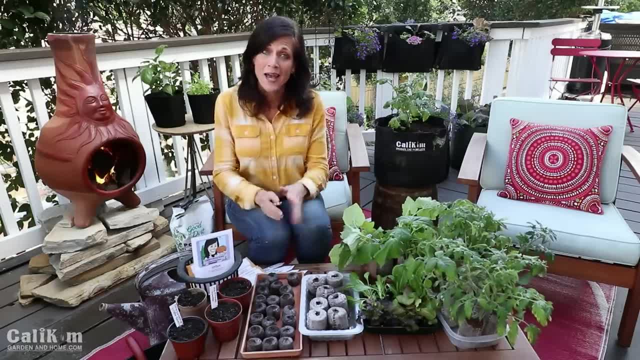 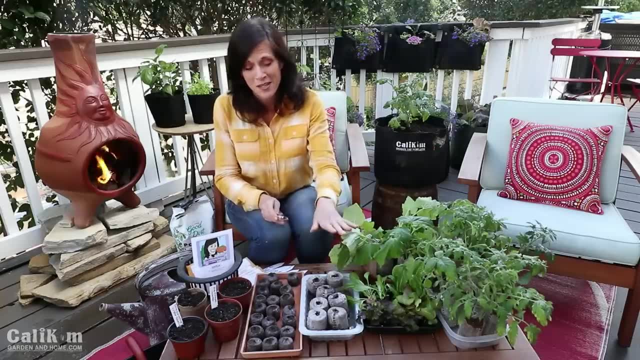 in your garden. We've got our squash and our cucumber seeds planted. The next category we're going to move on to is the seeds that you can get planted out in your garden very early, And that would be the greens and the peas, So we're going to plant those in the small-sized peat. 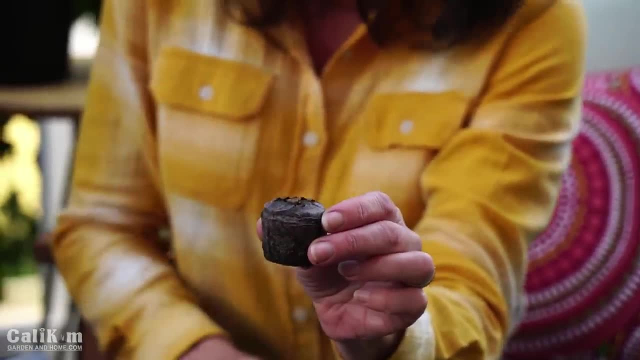 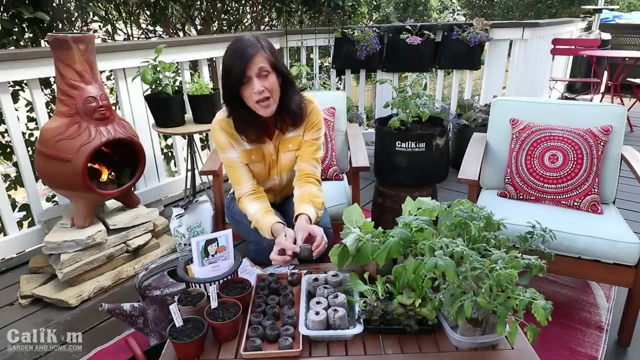 pellets because they're just going to be in here for a couple of weeks. These are also frost tolerant vegetables, So these are fun ones you can get planted outside before your last frost date. So these peat pellets have expanded. These small ones are. 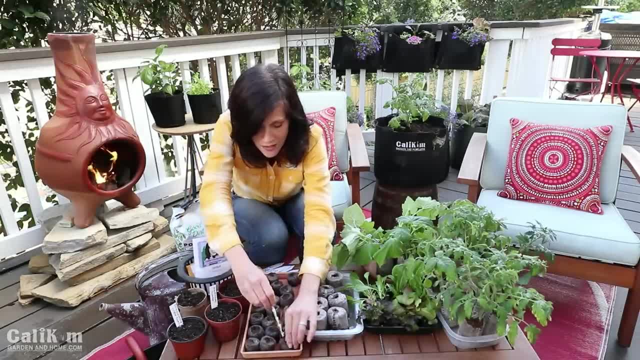 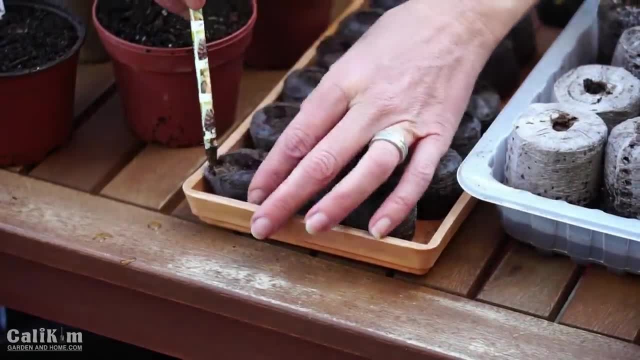 just about an inch tall. They're perfect for lettuce and greens and onions, And all you need to do to get things planted in the little peat pellets is just to peel apart the netting and fluff them up just a little bit with a pencil here, So just kind of loosen the soil a little bit. 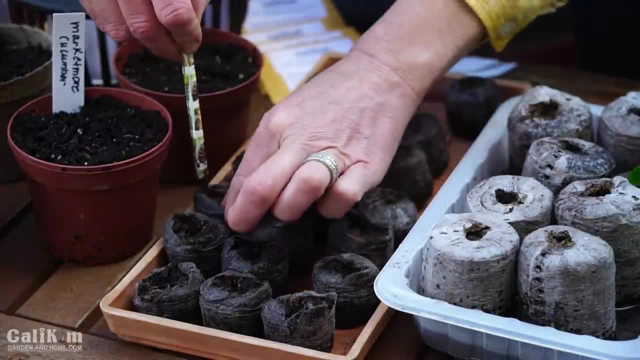 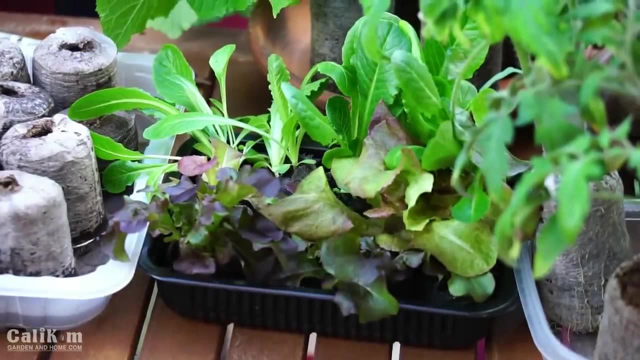 loosen the netting a little bit and we're going to drop the seeds right in the pellets. In just a couple of weeks you're going to have some beautiful lettuce seedlings that look just like this. So the two varieties we're going to plant today from the Spring Garden Seed Collection are the red romaine. 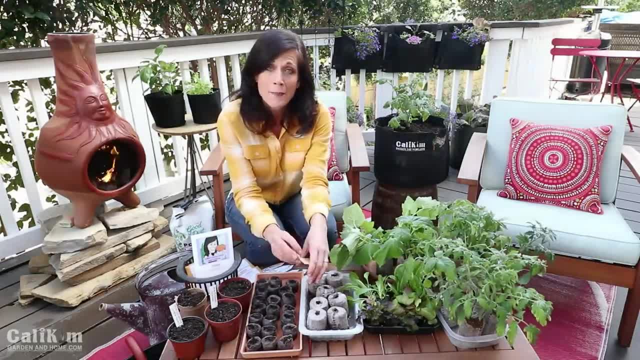 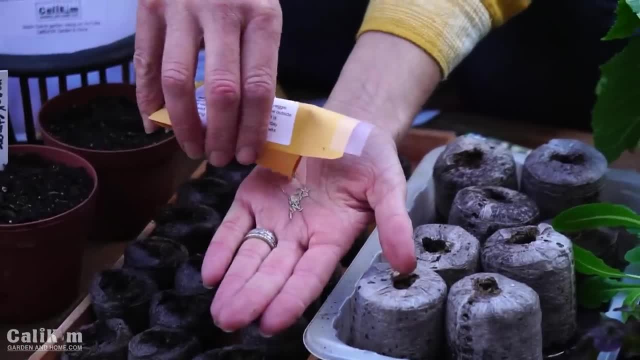 lettuce and the black seeded Simpson lettuce. Now I absolutely love growing my own fresh tasty greens. They're so delicious, so much better than store-bought and so so easy to grow. So if you've never grown your own salad greens before, you definitely want to get started with this. 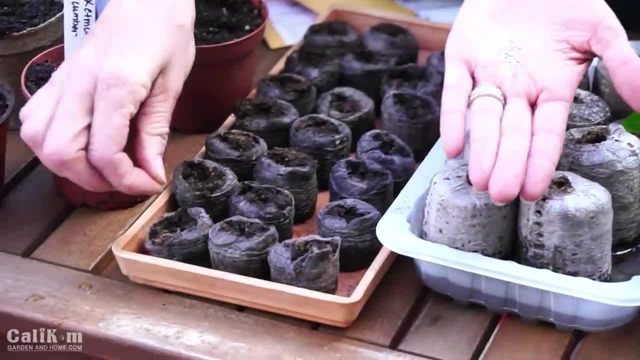 So I'm just going to take a couple of seeds- These are the red romaine seeds- and I'm going to drop a few seeds in each pellet. Now don't be too worried. if you get more than a few seeds in each pellet, You can always go. 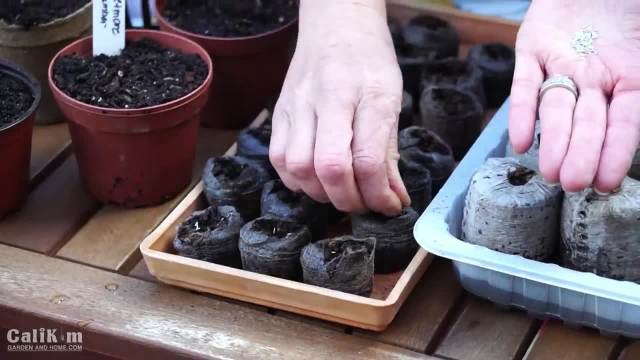 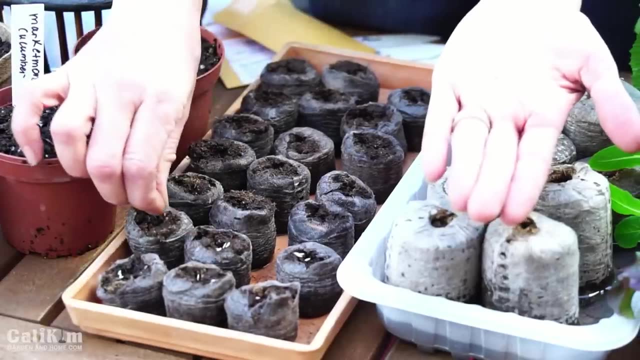 back out later and thin them out as they grow. But lettuce is a cool weather vegetable and it really likes temperatures under 75 degrees. That's why you want to get some lettuce started first thing in the spring, before the weather gets too hot. So we've got about six pellets there of the 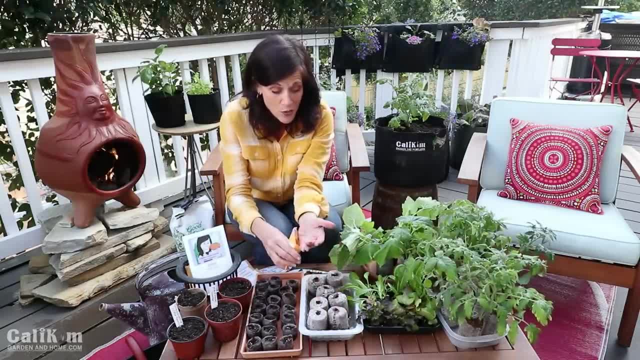 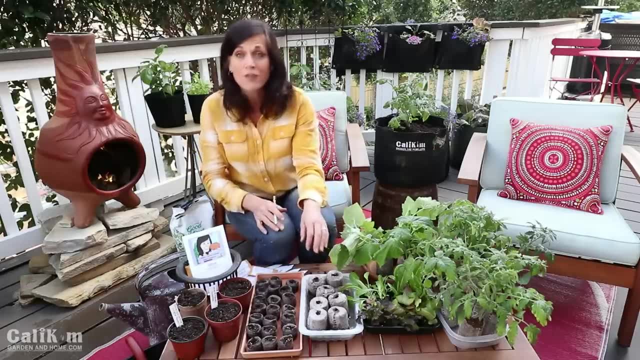 red romaine lettuce. And again, by doing So, we're planting our seedlings in pellets. We're avoiding the first mistake of using our garden soil. We're also going to avoid the second mistake of planting our seeds too deep. Lettuce seeds are. 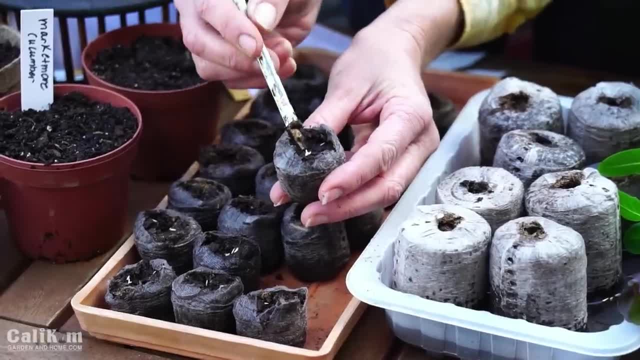 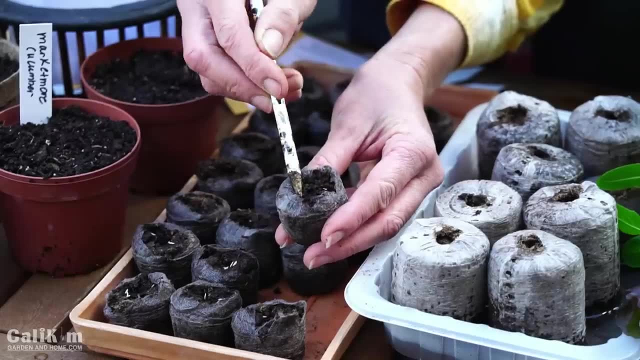 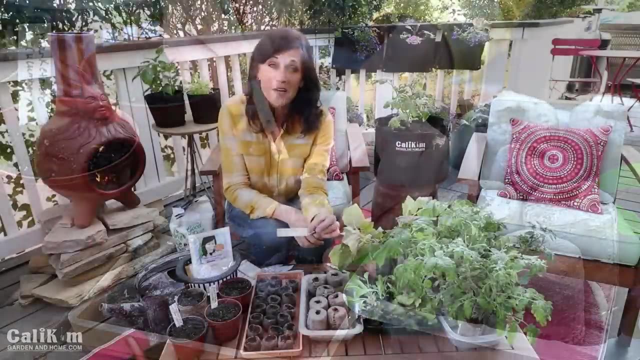 super, super, super, super small. So we're just going to put them on the top of the soil and barely press them down here into the pellet, And that will give them a much better chance of germinating. And then we're going to avoid mistake number three and we're going to go ahead. 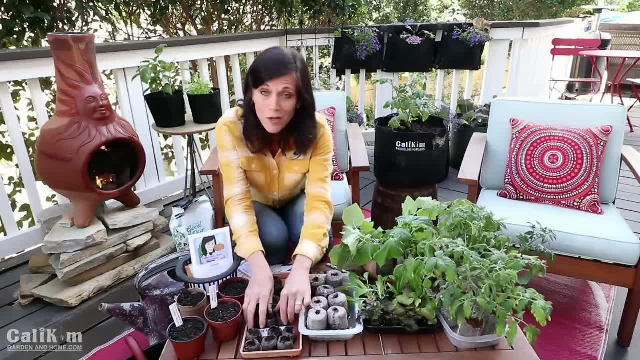 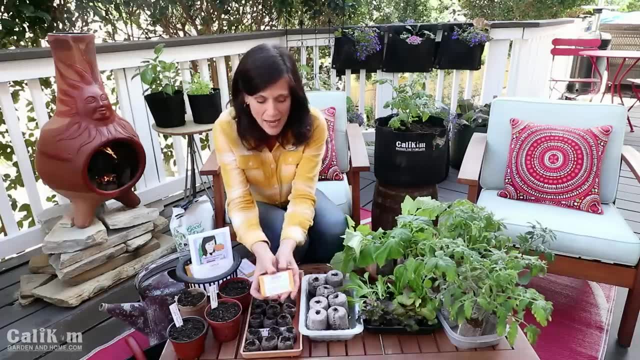 and plant them in pellets. So we're going to plant them in pellets And then we're going to label the red romaine lettuce. Red romaine is an absolutely beautiful variety of lettuce. you guys, You definitely want to grow this variety. The next variety I'm going to plant here is the black seeded. 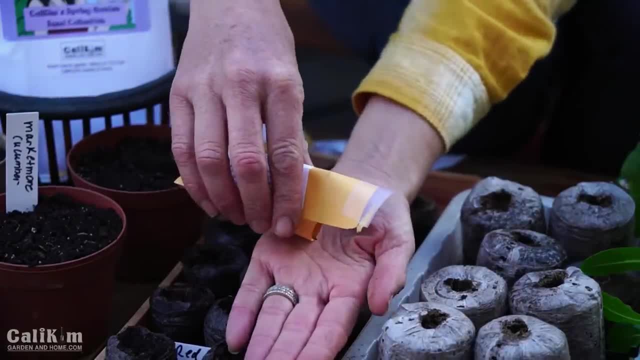 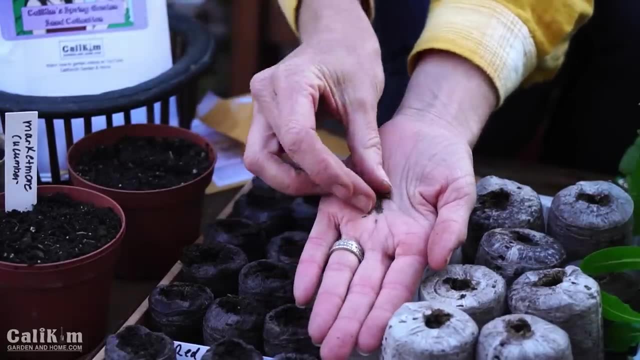 Simpson lettuce. And this is a nice fluffy green, bright green type lettuce. It's also more heat tolerant variety. It usually does well in temperatures of up to about 80 degrees. So you can see here the seeds are a black color. I'm going to plant them exactly the same way in the pellets. 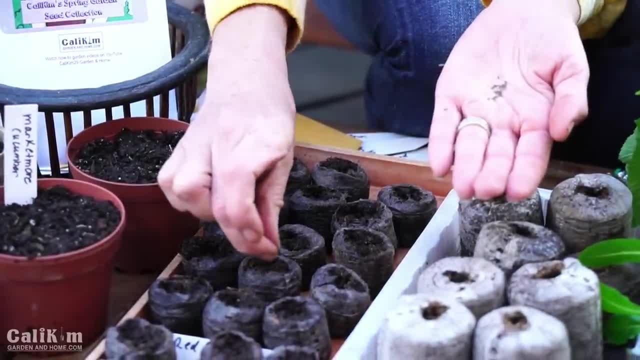 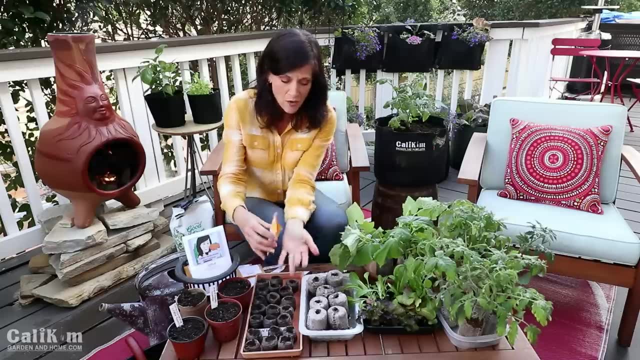 Lightly cover them up and label them and we are good to go. Next, we're going to plant our red Russian kale. If you have never grown kale, it's a super food. It's super, super easy to grow and it's a beautiful, beautiful plant, ornamental as well as edible. You can see the seeds. here are 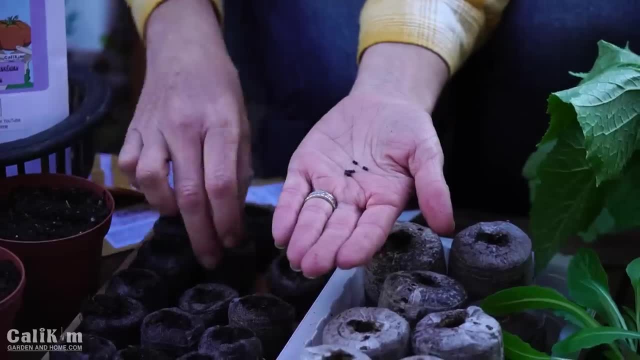 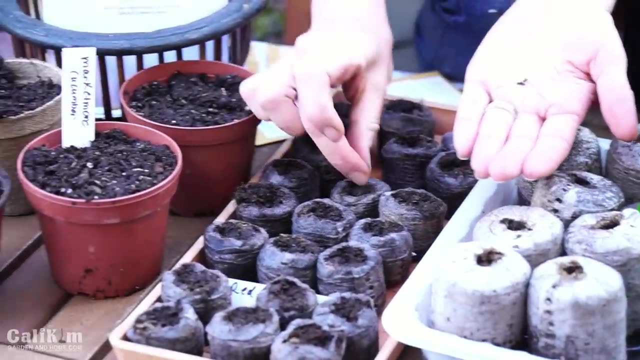 a little bit bigger, but I'm just going to plant one row of kale here because we're going to save a couple more pellets here for our onions. So I'm just going to drop a couple seeds in each pellet, cover them up, label them and we are good to go. 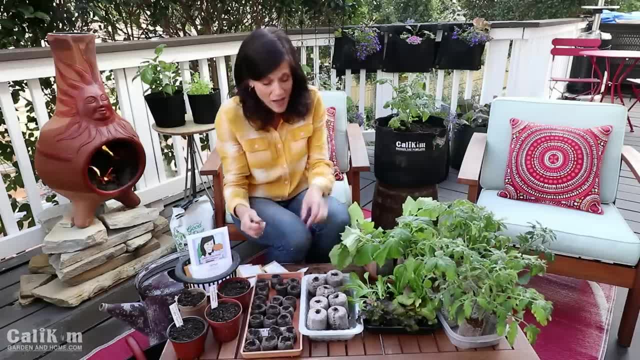 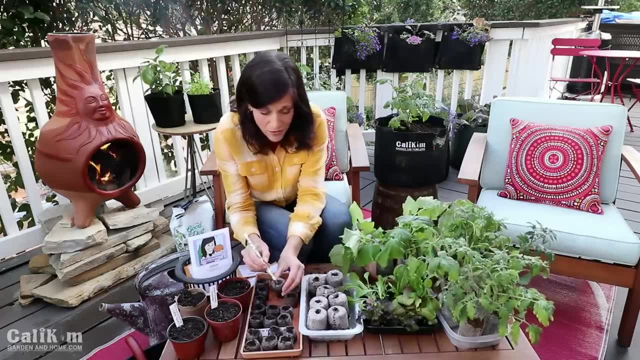 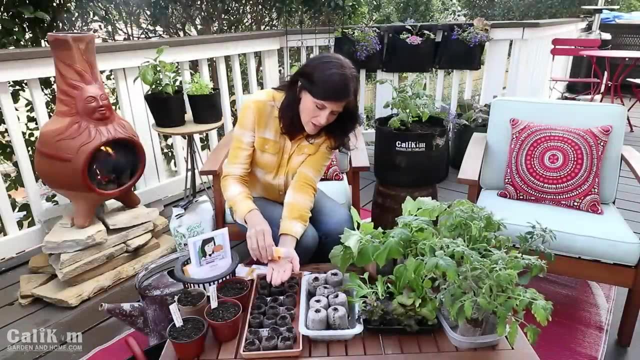 You're going to love having kale in your garden. It's so delicious in smoothies, great in salads. You're going to feel so good about feeding kale to your family. it's just so, so tasty. And next we're going to plant our bunching onions. These are so much fun to grow. 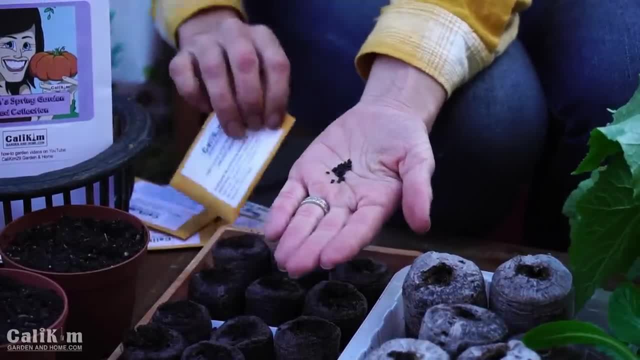 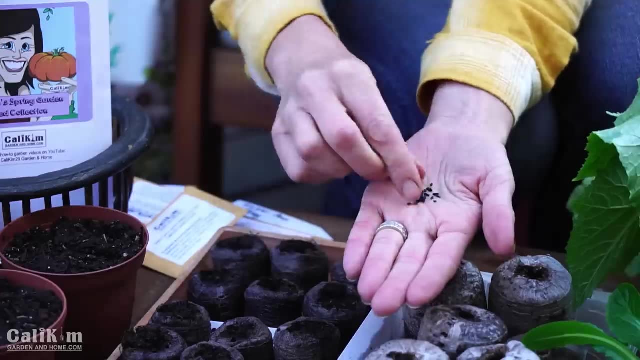 These can be harvested when they're very, very small and out in soups, salads or cereals. This group here I fashioned a bunch of garlic. So the unfold here and how you and just use to flavor recipes. you can see the seeds are pretty small. drop a. 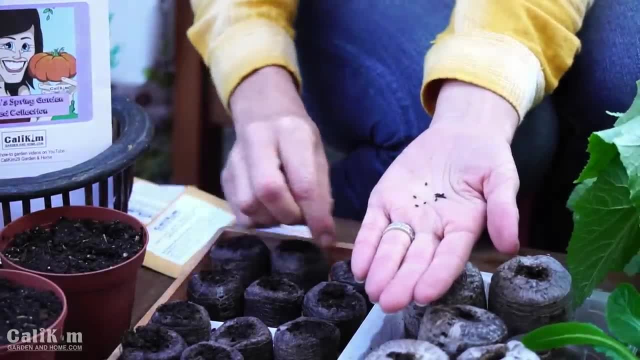 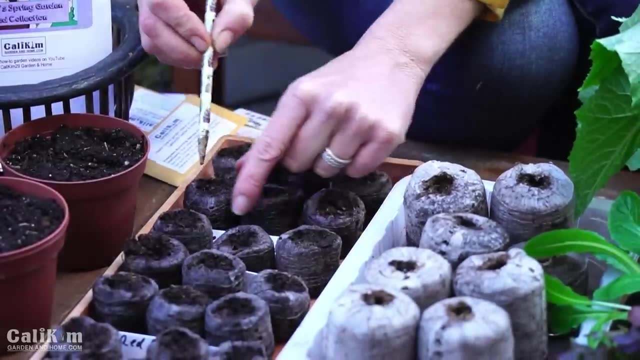 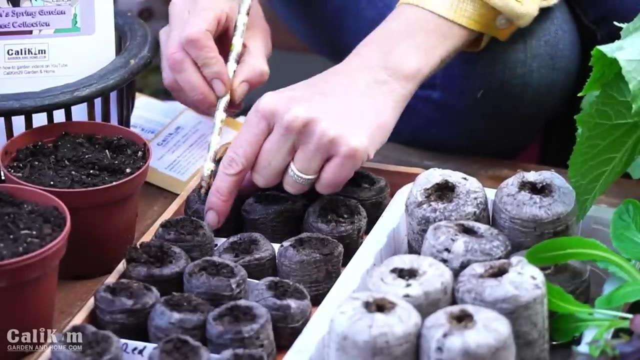 few in each pellet, cover it up. we're ready to go. you guys are getting this down now. it's so, so easy to start your seeds indoors and so much fun too. so I would encourage you, grab your kids, grab a friend, and get yourself some seed started now, along with your greens and your onions- the other vegetable you can. 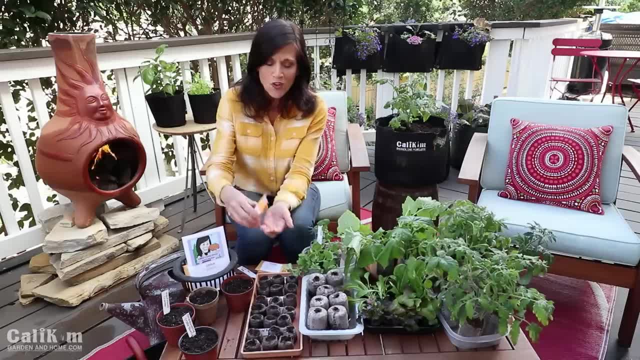 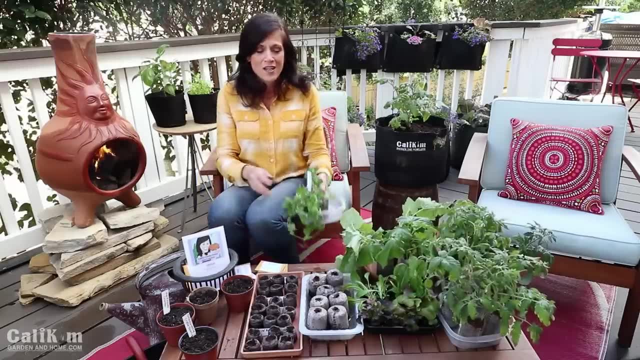 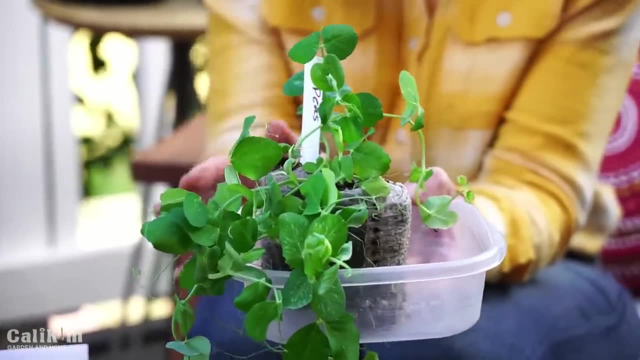 get planted very early in the spring, while the weather is still cool, is sugar snap peas. you've never grown sugar snap peas before. you are in for a treat- super, super sweet, tasty. a lot of times, guys. honestly, my sugar snap peas never make it inside. there's so much fun to snack on in the garden. now pea seeds are. 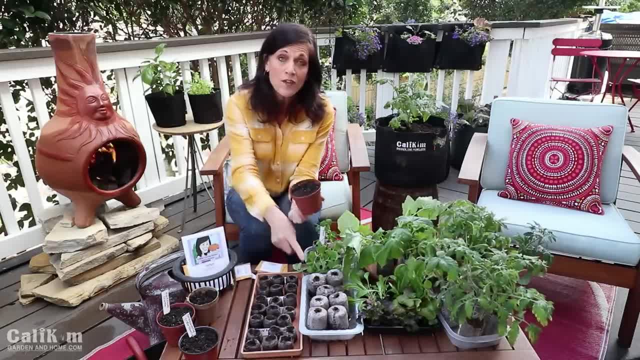 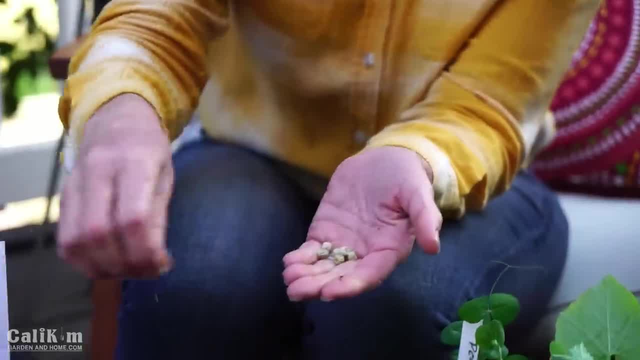 another one of those seeds I like to plant in the cups with soil or in the large peat pellets. if you plant them in the smaller size peat pellets they outgrow them very quickly. so I'm just gonna poke a couple of pea seeds down into the soil here. just poke them down in about a half inch or so, not way. 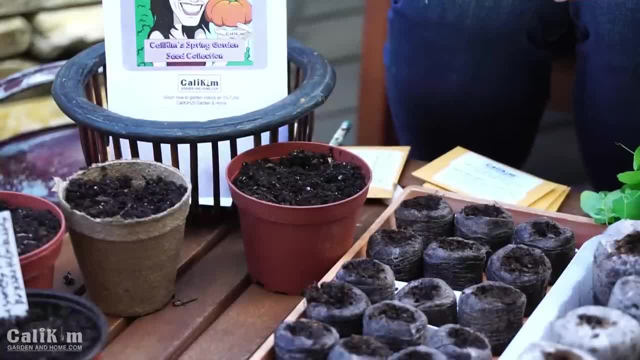 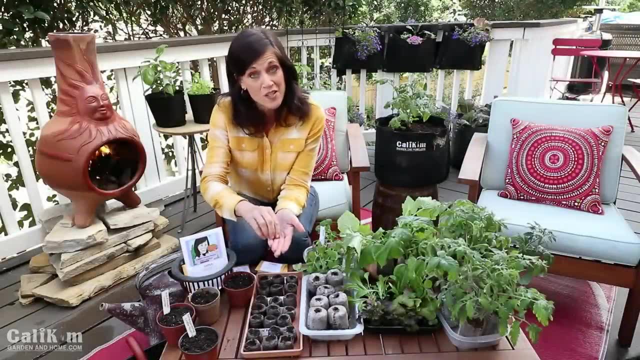 down into the bottom of the cup. that way they'll germinate quickly and you'll be planting these pea seeds out in your garden about two to four weeks from planting your seeds indoors. pea seeds are one of those vegetables that can even take a light frost, so you can get them going inside now and then plant. 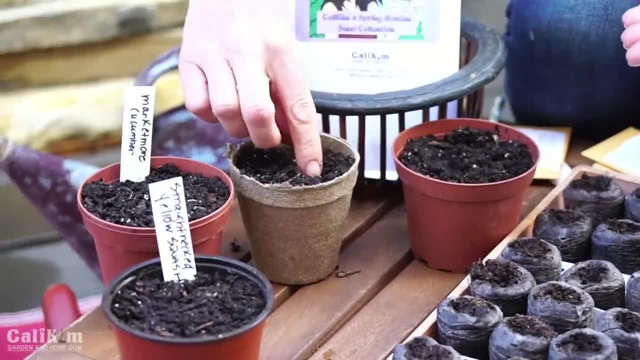 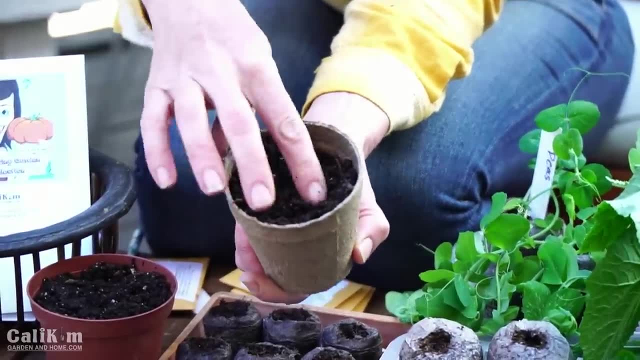 them out in your garden even a couple of weeks before the last frost date, as soon as it's thawed. so I'm just going to poke these here down into the soil and they are ready to go. of course, we're not going to forget to label them, right. 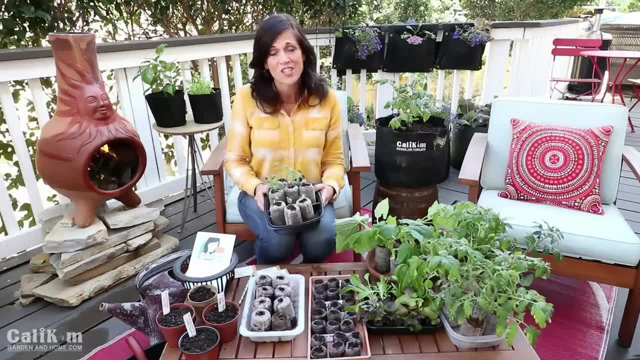 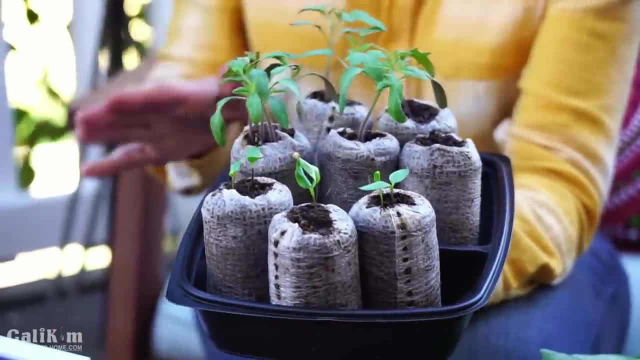 now, the next category of seeds we're going to start from our spring garden seed collection are tomatoes, peppers and basil, and I'm going to start these in the larger size peat pellets because they're larger size vegetables and I don't want to have to transplant them again. 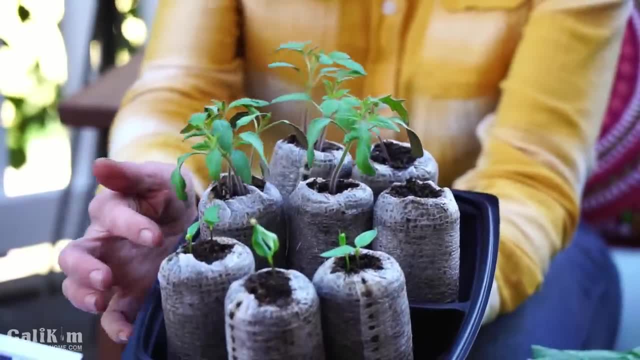 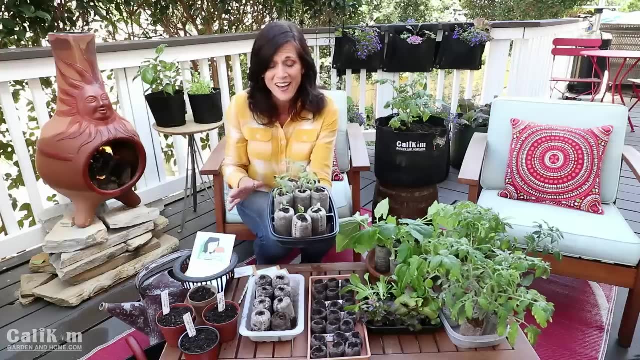 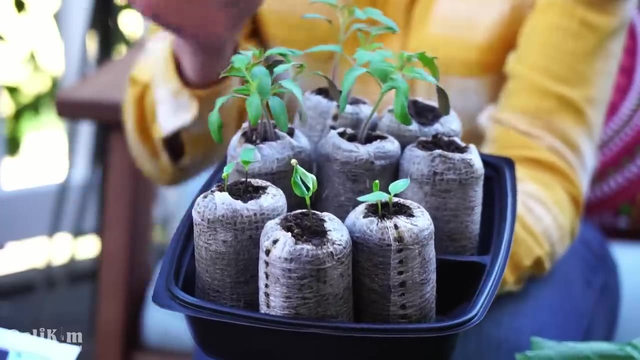 before I get them planted outside. so here I started these tomatoes and peppers. these are actually from my salsa garden seed collection. started these exactly two weeks ago. so just think, guys, start your seeds today. in about two weeks you're going to have some beautiful tomato and pepper seedlings that look just like this, and I'll show you exactly what to do. 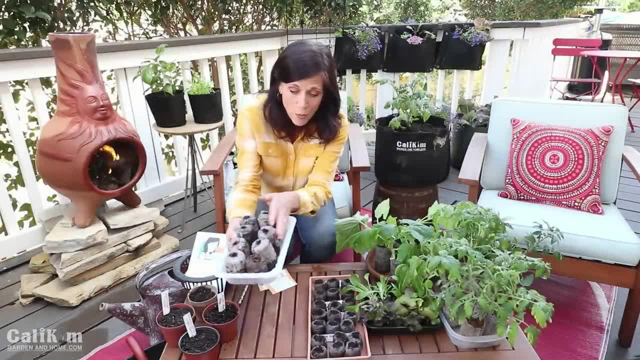 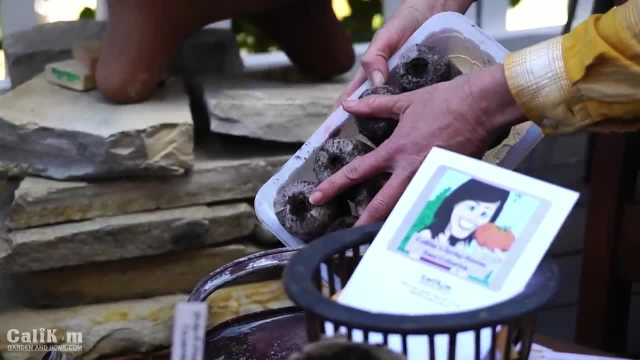 now there is just a little bit of water left here in the tray. I am going to go ahead and pour that water off into my watering can here, because we are going to talk about mistake number three in just a minute and that is watering too much, so we'll get to that in just a second. 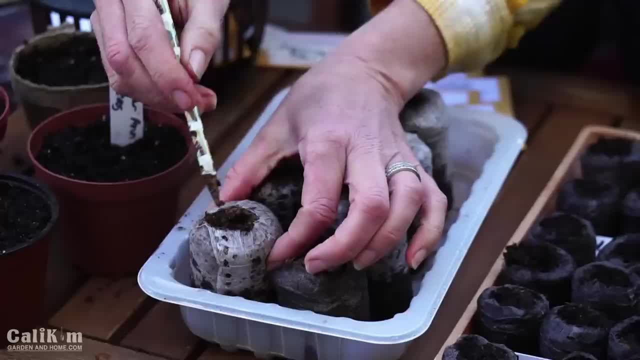 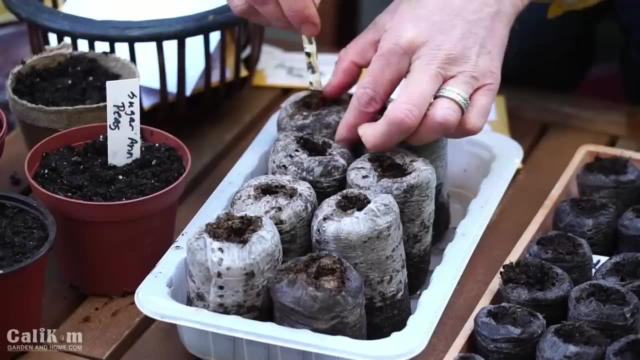 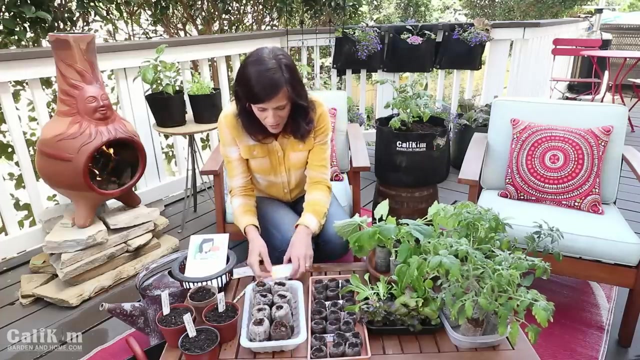 so I poured out the extra water. I'm going to go ahead and peel apart my netting and fluff up my soil, and the first variety we're going to plant is a beautiful Golden Jubilee tomato. this is a super, super sweet tomato, gorgeous and yellow, all America selections winner. so it's going to be very, very 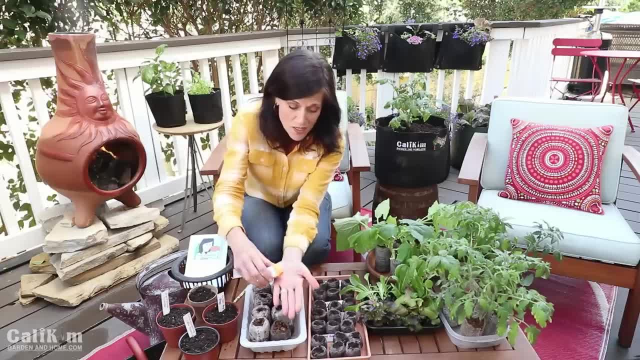 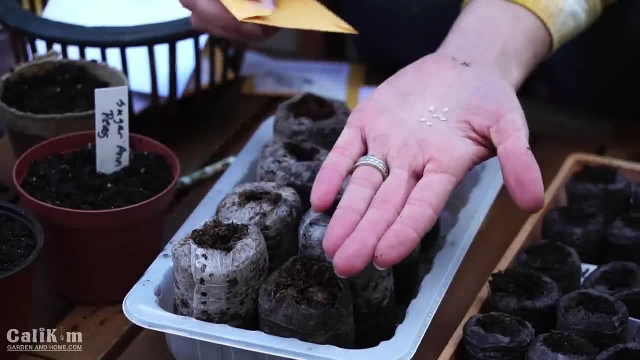 productive in your garden. you're going to absolutely love having this Golden Jubilee tomato in your garden, so I'm going to pour into my hand about four seeds or so. there we go, got a few more than four, but that's okay and I'm going to drop just a couple of seeds. 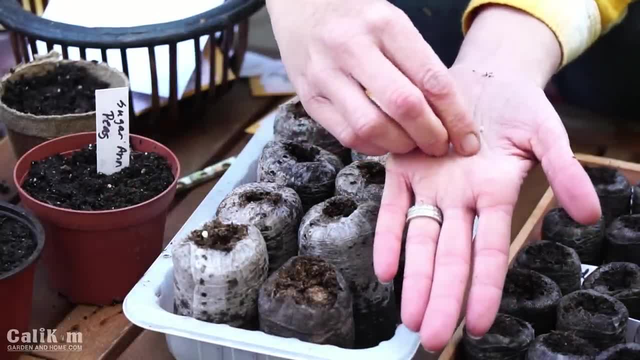 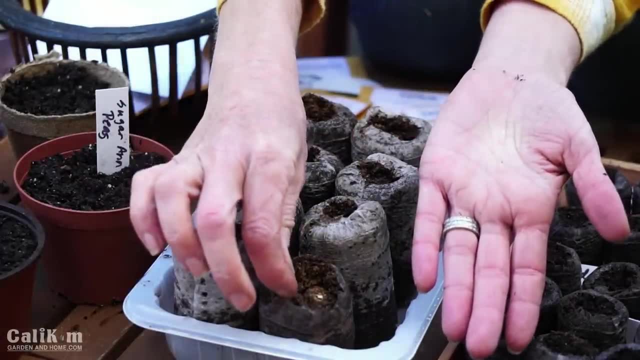 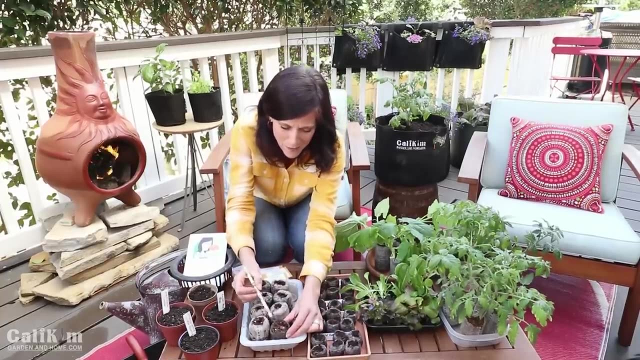 into each pellet. I'll do three seeds in each pellet. just drop it right there on the surface. I've got a fourth seed, so I'm going to throw that in there too, why not? don't be afraid to experiment in the garden, guys. it's always fun to see what happens when you experiment, and I'm going to poke those down. 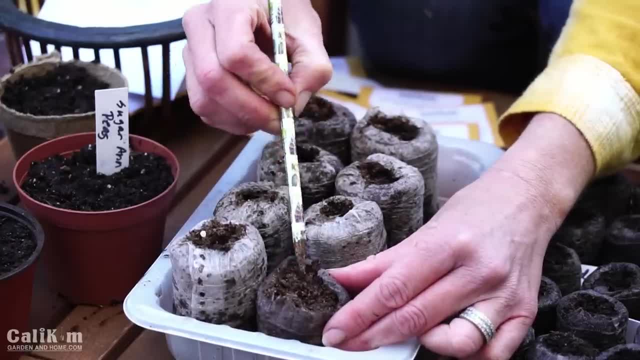 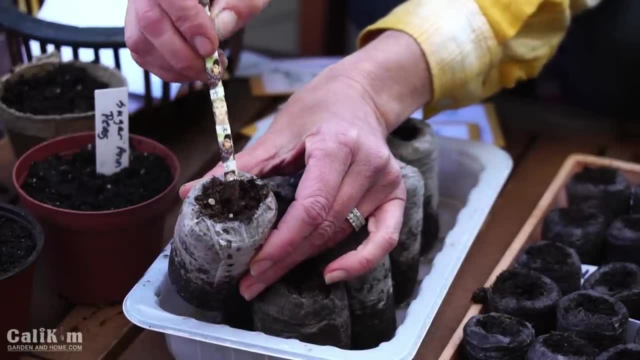 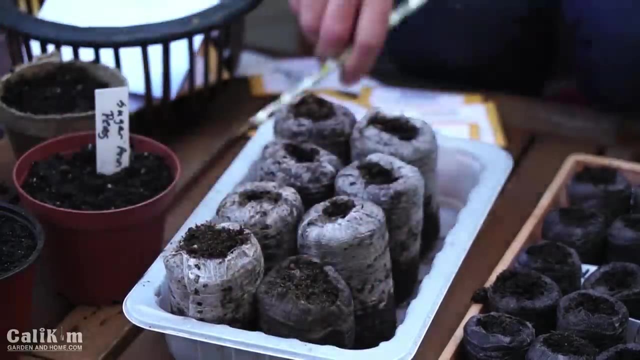 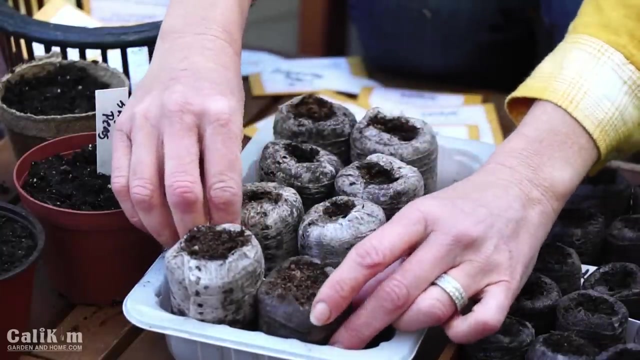 into the pellet here again, very lightly cover it with soil, not going to make the mistake of planting them too deep. I'm going to pop in my label. we're really getting the hang of this now, guys. there's really not much to it. it's super quick. 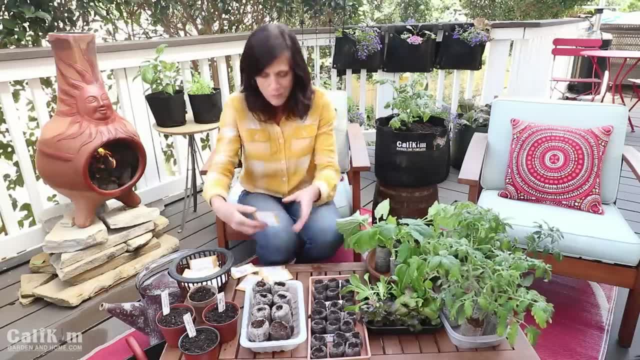 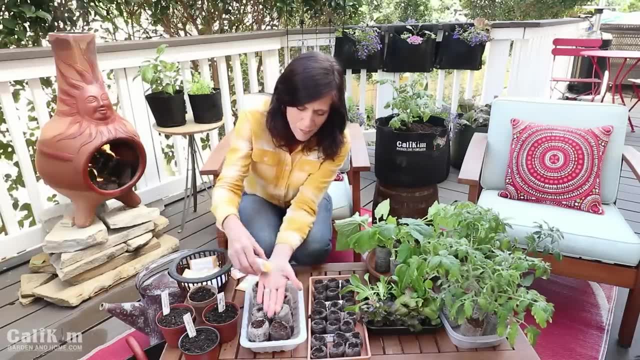 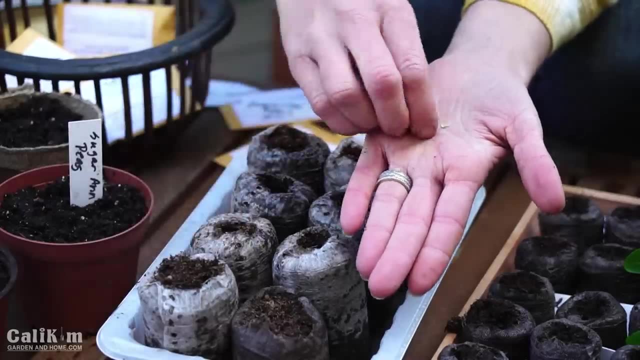 and simple and gets your seed started. so the next one we're going to plant is the maraglobe tomato. this is a beautiful, nice red slicing tomato, very prolific. it's going to be a lot of fun to grow in your spring garden. so I've got five seeds. I'm going to plant two or three in each pellet. 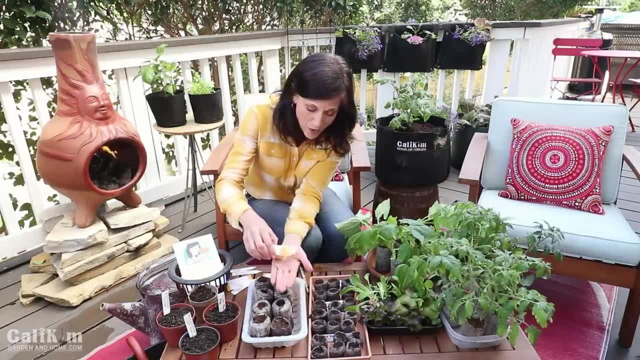 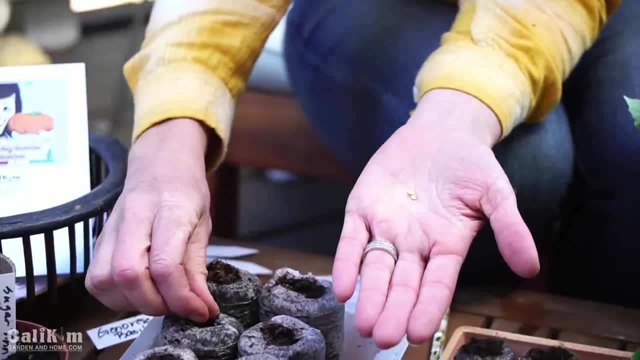 next, we're going to plant our California Wonder and our Hungarian hot wax pepper. we're going to do it the exact same way, so once you get the hang of it- so easy starting from seed indoors. So I'm going to plant one pellet each of the Hungarian wax. 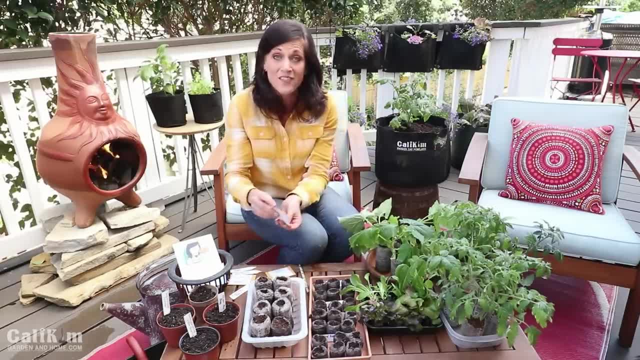 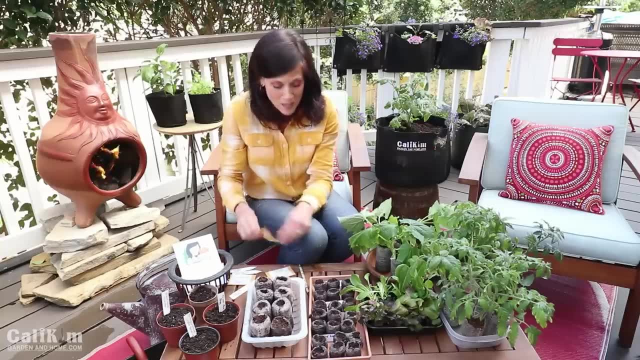 and one pellet each of the California Wonder, because I've got two pellets left here and that's what I'm going to use to plant my basil. It's going to be so much fun to grow these indoors and watch the seedlings pop out from the soil. You're going to get such a thrill from that. 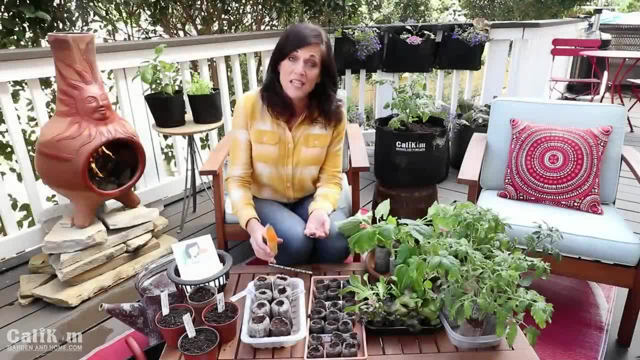 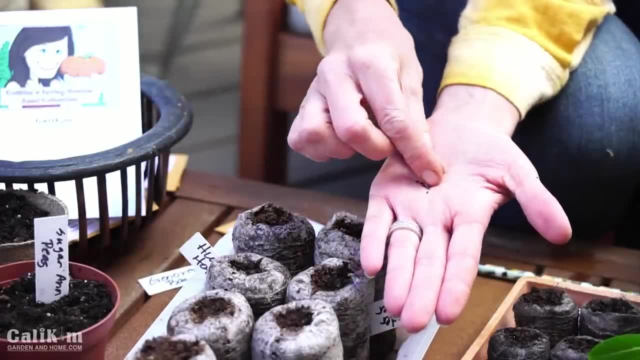 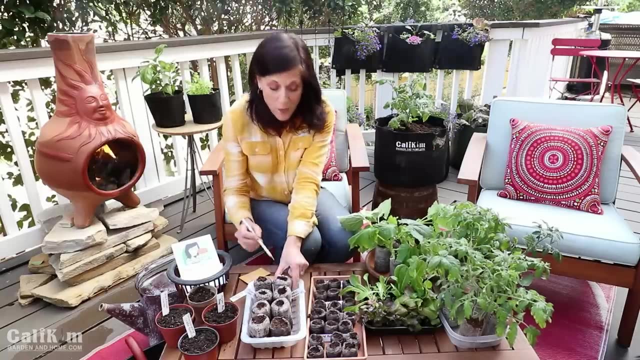 I promise you Now I'm saving the last two pellets here for my basil. The basil is a really tiny seed and I'm going to pop about three seeds in each pellet. Now, basil can also be direct seeded right in your garden, but it's always fun to get some going indoors and that way you have basil to plant. 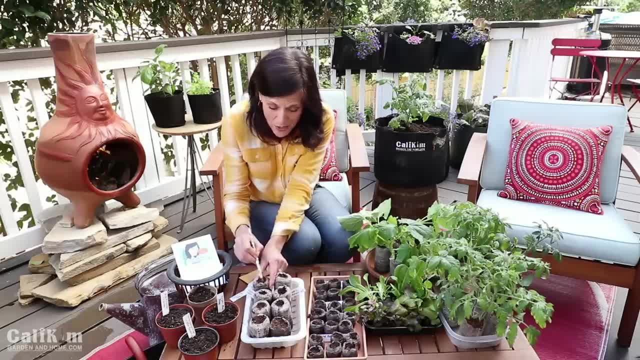 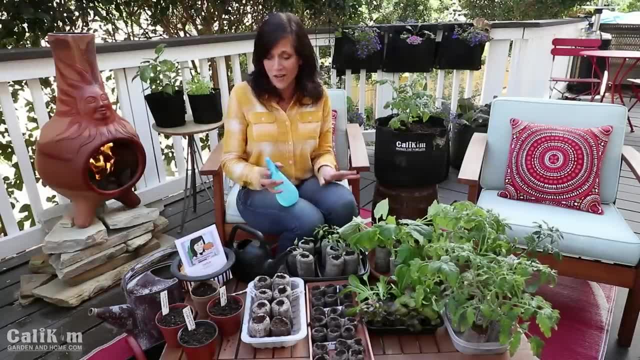 outside as soon as the weather is warm enough, and you can always pop more seeds out in your garden later. The fourth mistake a lot of people make when starting their seeds indoors is about watering. Now, when we first start our seeds, we're just going to lightly spray them and mist them with. 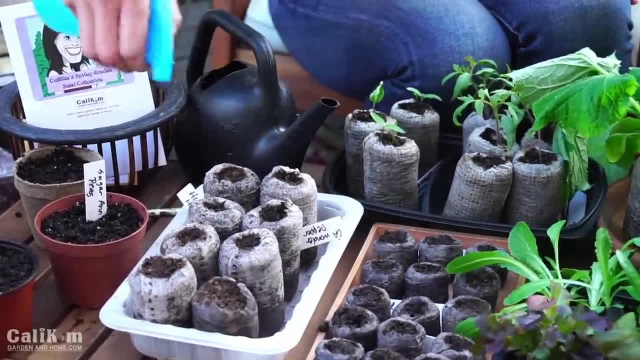 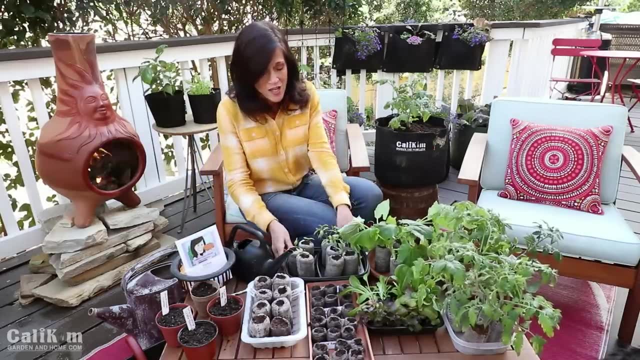 a spray bottle just to get the seeds kind of settled down in there. But you don't want to over water your seedlings As they grow. you want to be really careful about not soaking them down too much and you want to make sure you water from the bottom. 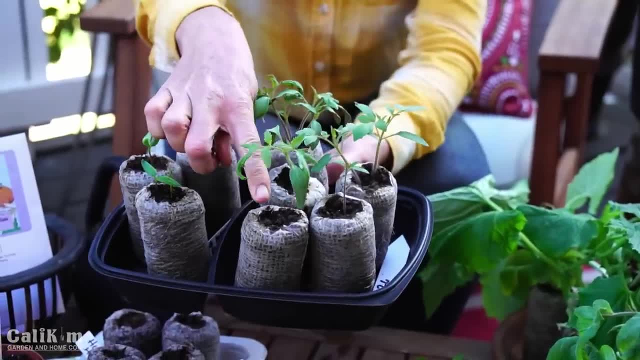 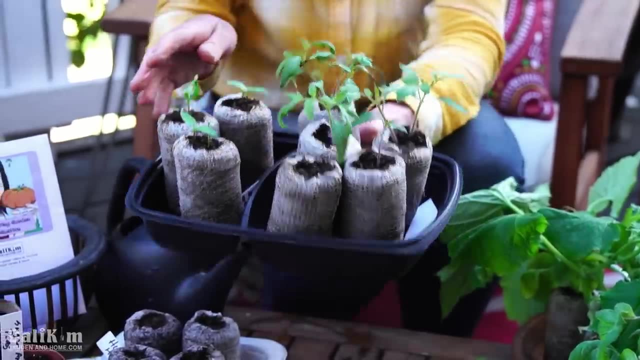 So these seeds again. I started a couple of weeks ago. They don't need watered right now because you can see how the top of the soil is a dark brown color. That's a sign that the soil has plenty of moisture. When they do need watering, as they grow they will turn a lighter brown color. 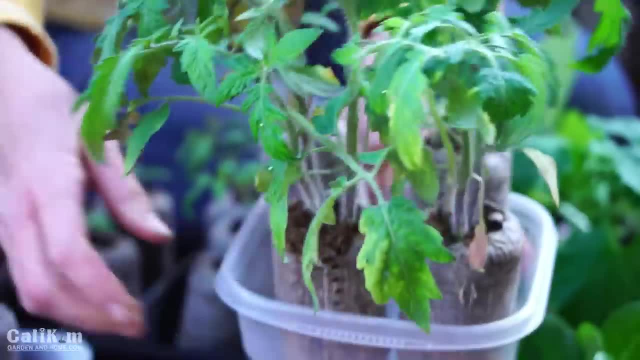 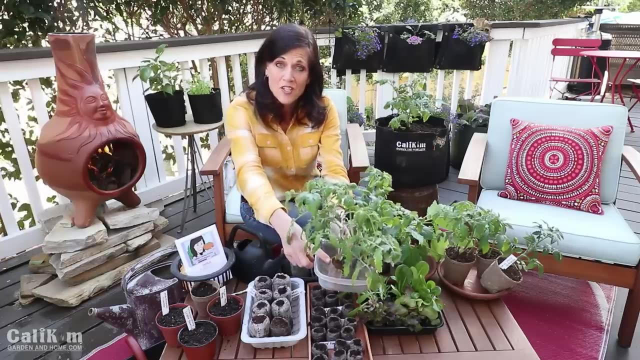 like these little tomato seedlings are right here. You can see how the top of the soil is lighter brown than this pellet here, and the lighter brown color is an indication that they need water. Now, when they do need water, water them from the bottom. So I'm just going to water. 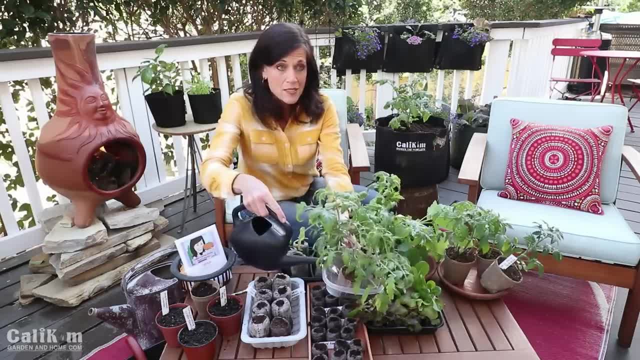 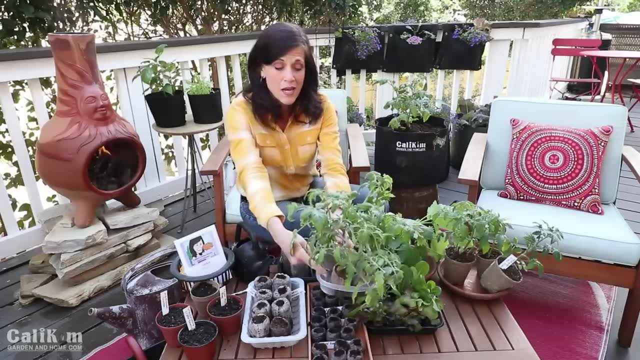 here from the bottom. Let the pellets soak up the water, and when the top of the soil turns a dark brown color, that's a sign that all the pellets have absorbed the water that they need and you can dump the extra water out. So don't make the mistake. 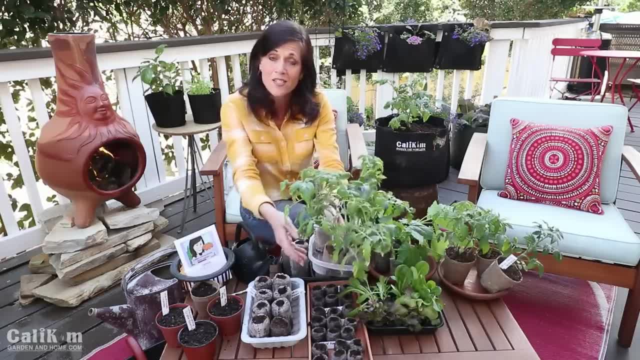 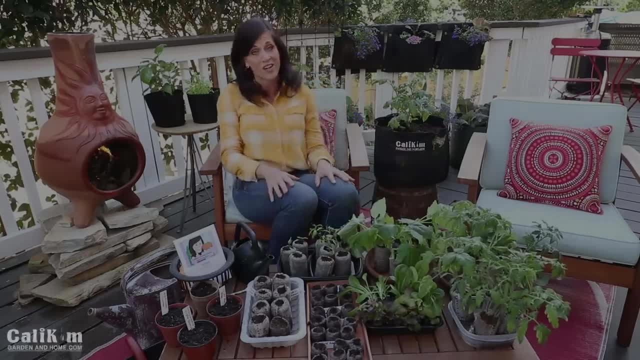 of letting your pellets sit in water too long, because that tends to rot the roots and you don't want the soil super, super soggy, You want it just an even amount of moisture. The fifth mistake a lot of gardeners make with starting seeds indoors is light. 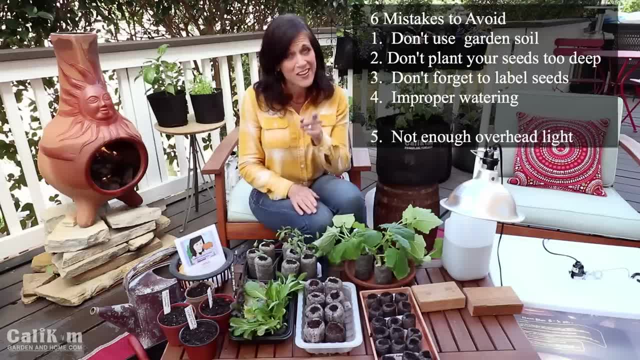 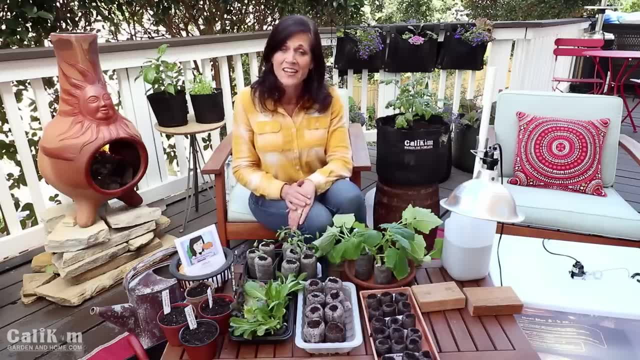 not enough overhead light. Now I know what you're thinking: grow these in a sunny windowsill, right? No, oftentimes a sunny windowsill, even if it's south facing, doesn't provide enough overhead light for your seedlings, because you know what's going to. 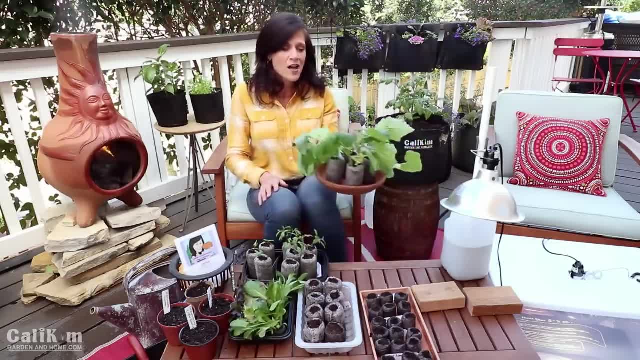 happen is Your seedlings are not going to have enough overhead light. You're going to have to use a light bulb that has the right amount of lumens and kelvin for growing plants. I've got two simple setups that you can do to easily grow your seedlings indoors. 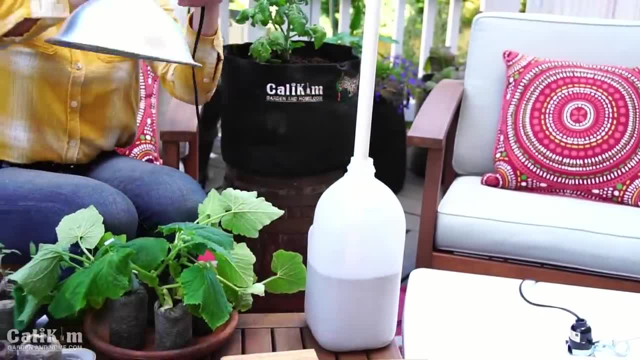 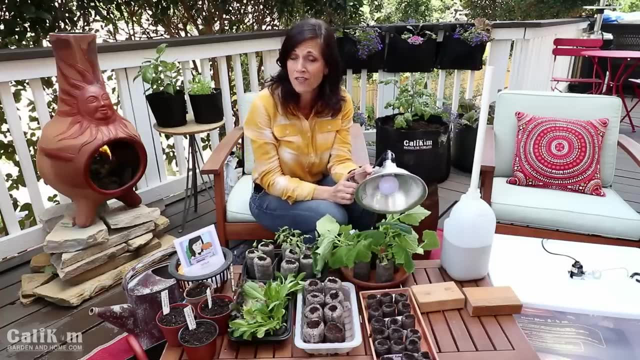 They both use this clamp light. You can pick up one of these clamp lights at pretty much any hardware store, and you do need to use a special light bulb that has the correct amount of lumens and kelvin for growing plants. Lumens simply refers to the brightness or the intensity of 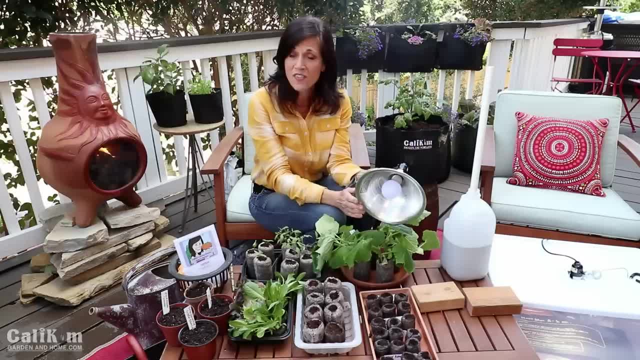 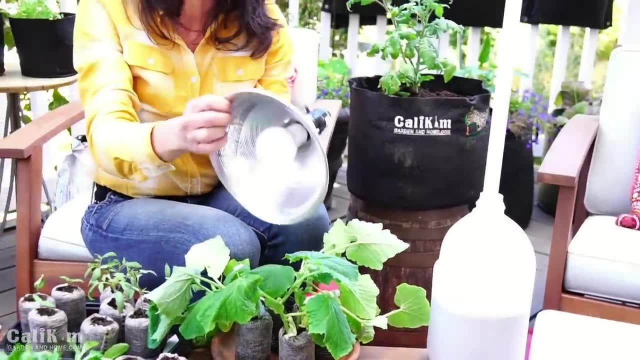 the light. You want to choose a light bulb that has the lumens between 1500 and 3000. Because that will provide your seedlings with super bright, intense light. You want your light bulb to have a kelvin between 4500 and 6500, because those are the numbers that will mimic. 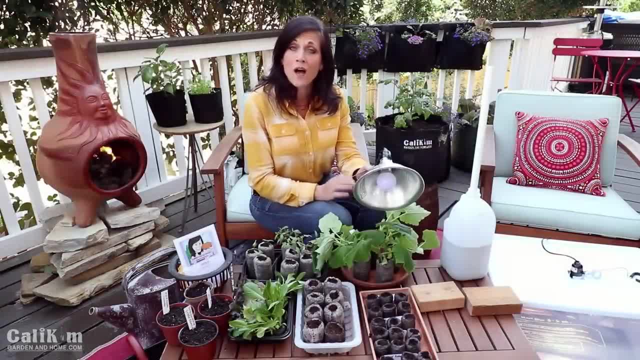 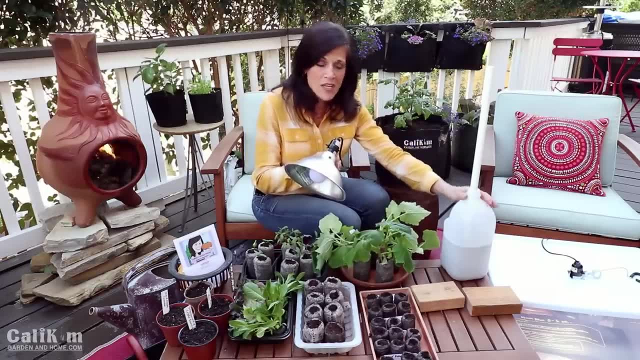 daylight, So I'm going to put links to everything in the video description below and also a link to a video that tells you how to do this in more detail. Now you can get this clamp light set up in a couple of very easy ways On this gallon jug filled with sand, PVC pipe stuck in the middle. 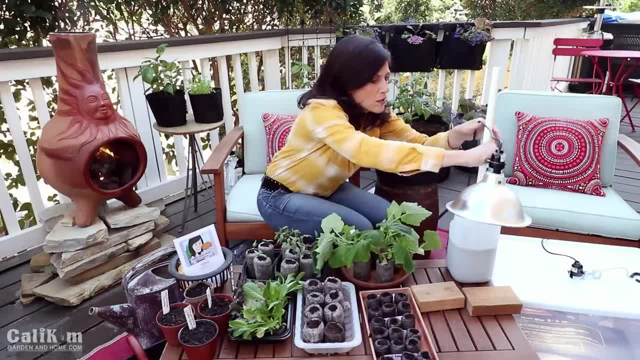 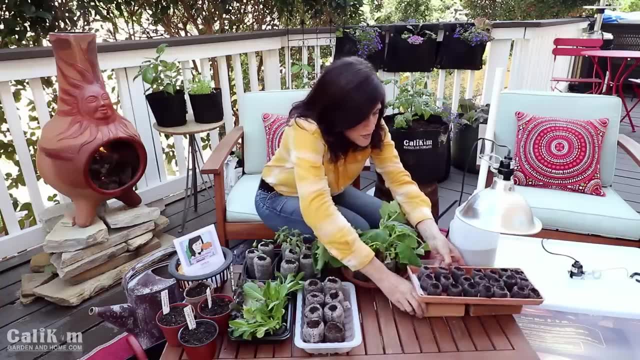 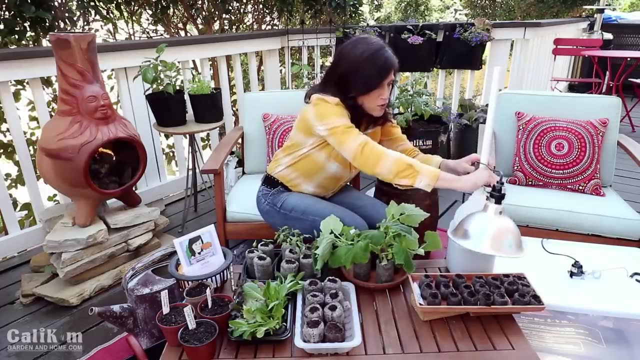 to provide it with some stability, And you just simply clip your clamp light onto the PVC pole, You place your seedlings right underneath And you always want to make sure that your light is no more than two inches away from your seedlings, So it's really important that you be able to control the height of the clamp light. 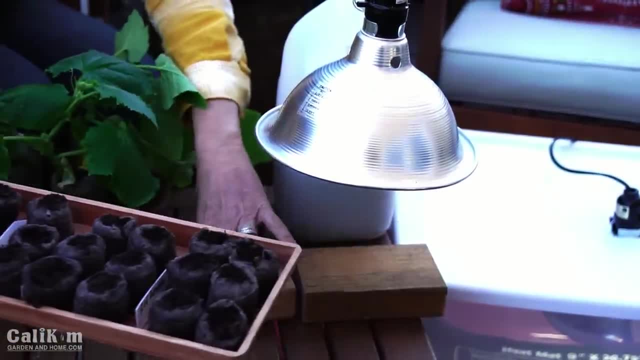 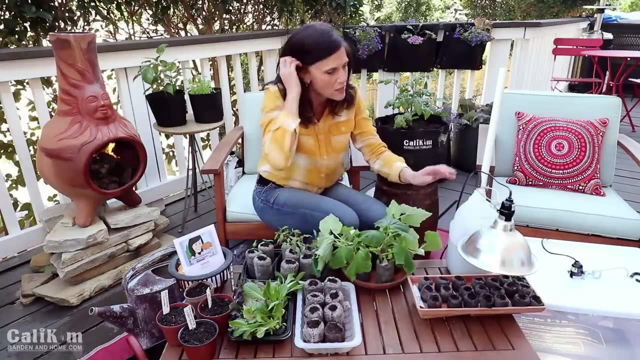 You can either move it up and down the pole or you can also put things underneath to raise and lower the seedlings as they grow. So you're going to put these lettuce seedlings right underneath this clamp light And we're going to leave our lights on. 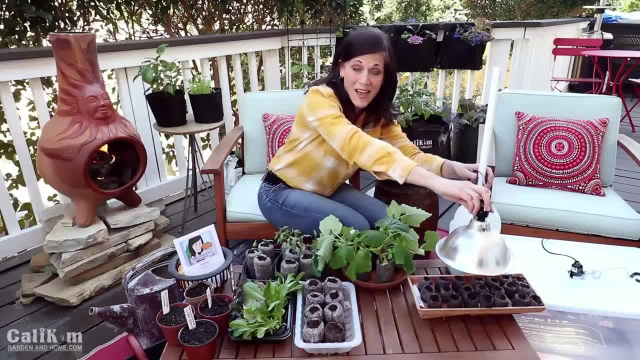 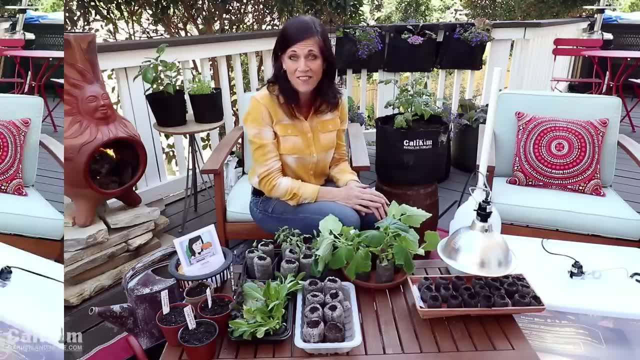 For 16 hours a day and off for six hours a day, And I love to hook them up to a timer so that it totally takes the guesswork out of it. You don't have to remember to turn your lights on and off. The second super easy setup for growing indoor plants: a lot of you have already seen this. 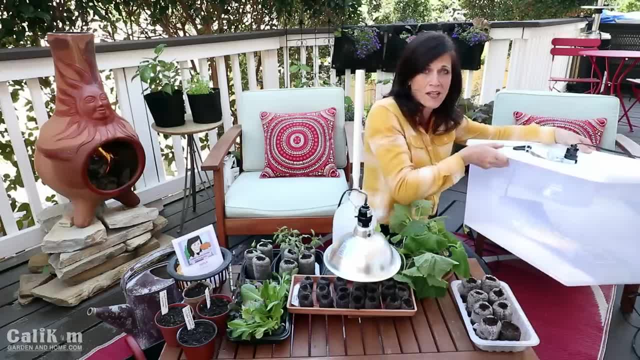 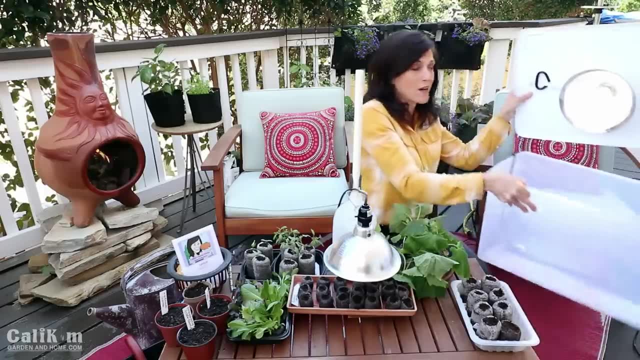 is the grow light box. I absolutely love this. It's super, super handy. Gary, over the rest of garden, invented this. It's a wonderful way to grow. So inside this plastic bin, here is another one of those clamp lights And I'm going to put this on the top of my plant And I'm going to put 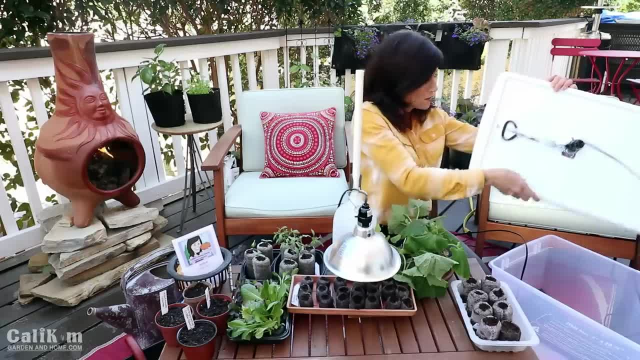 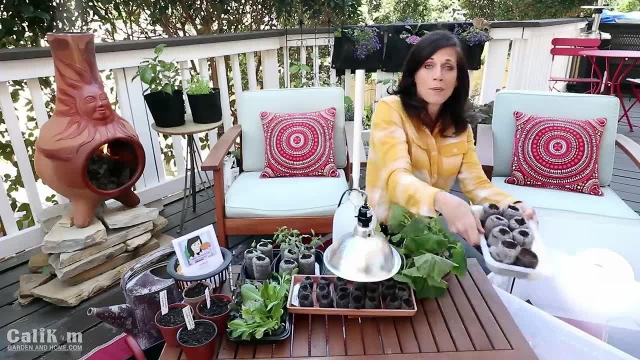 this on the top of my plant And it's hooked onto the top. Just cut a little hole in the top, hook the light right on here And then you just place your seedlings inside. Now these are the tomato, pepper and basil seedlings, And the key to getting pepper. 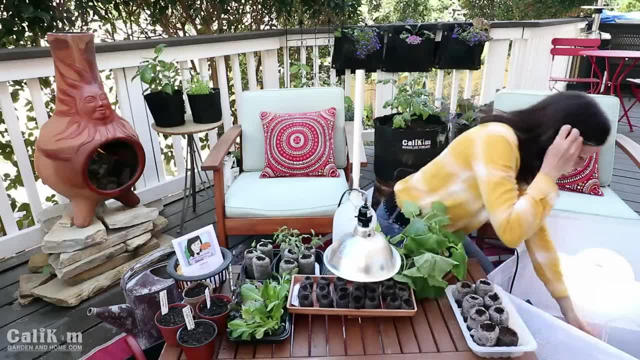 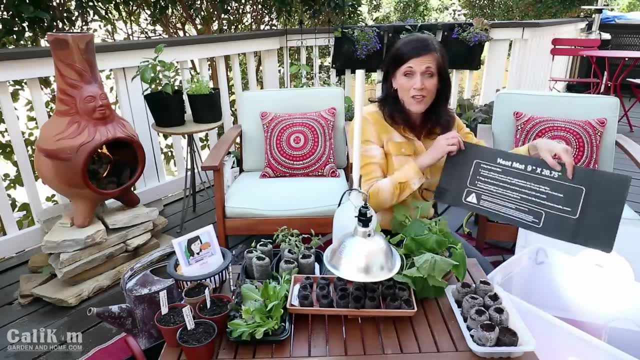 seedlings to germinate is a heat mat. So inside this grow light box I have a heat mat And it's also very beneficial to tomato and basil seedlings, Although they don't absolutely need the heat mat to germinate. it is very helpful, But the peppers definitely need. 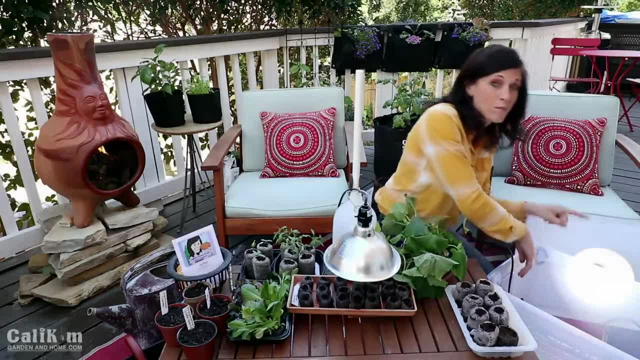 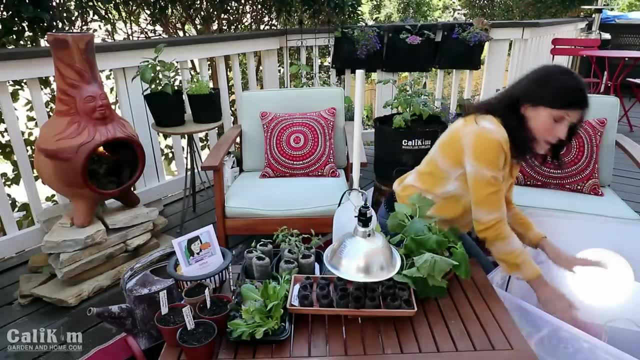 that bottom heat. So if you've ever had trouble getting peppers to germinate, the bottom heat is really the key. I'm going to place these seedlings inside the grow light box on the heat mat. I'm going to leave them on the heat mat until they germinate And then I'm going to put the lid. 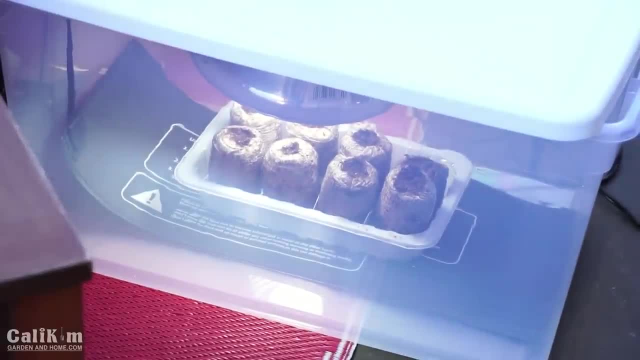 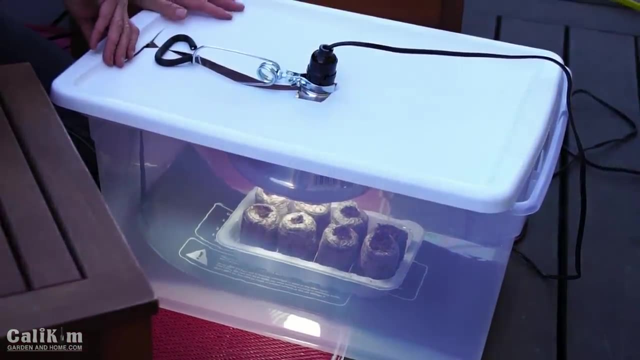 on And I'm going to leave the light on again, 16 hours a day on, 6 hours a day off, And that way the seeds are met with that bright, intense light as soon as they break the surface of the soil. Now I am going to leave this lid ajar just a little bit And then I'm going to leave this lid.